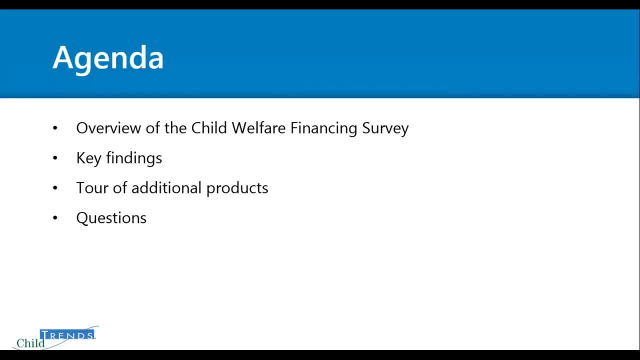 So, as for an agenda for today's call, we will first start off with an overview of the Child Welfare Financing Survey. Just provide some background about what that survey is. We'll go through the key findings from that survey. We'll also give you a little bit of background. 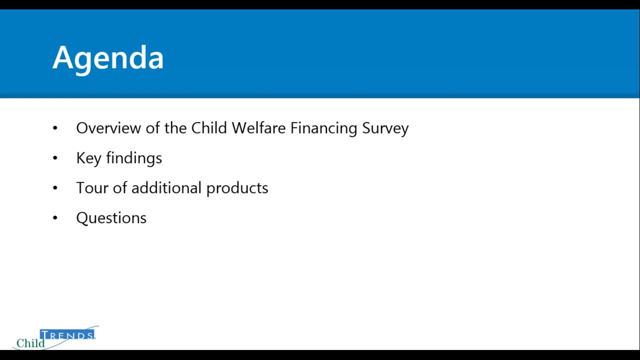 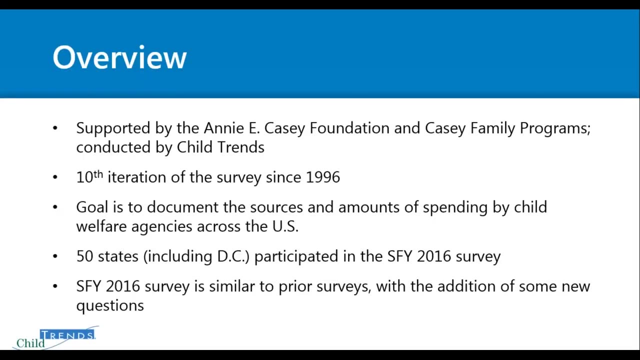 We'll also provide a quick tour of the products that we have related to this survey, that are available on the Child Trends website, And then, like I just mentioned, we'll have plenty of time for questions at the end. So, as for an overview of the survey, the Child Welfare Financing Survey is supported by the Annie E Casey Foundation and Casey Family Programs. 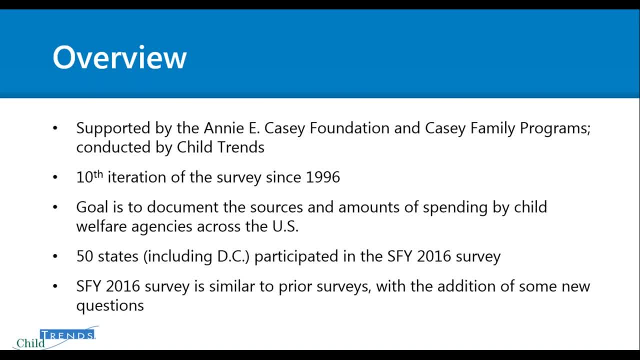 And it's conducted by us here at Child Trends. This is the tenth iteration. It's a state fiscal year 2016 survey. This survey is the tenth iteration of the survey since 1996.. And the goal of the survey is to document the sources and amounts of spending by child welfare agencies across the country. 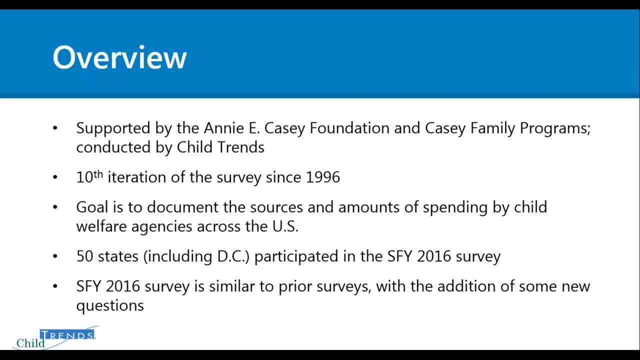 And data collected through this survey allows for documentation of national and state-specific trends, as well as comparisons across states. This year, for the state fiscal year 2016 survey, 50 states, including DC, participated. Unfortunately, Puerto Rico and Vermont were unable to participate this year. 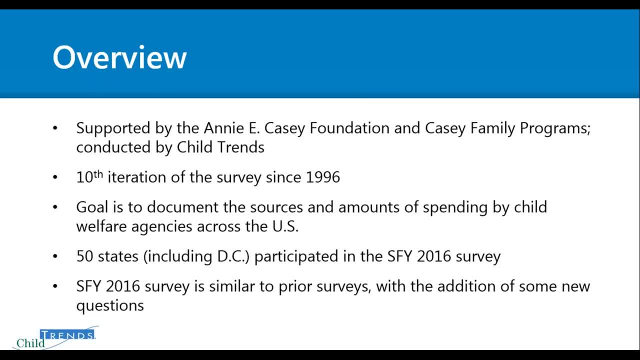 But when possible, we incorporated data from Puerto Rico and Vermont that they provide to the Department of Health and Human Services at the federal level. This allowed for some inclusion of data from some funding sources, but not all. So that's just one thing to keep in mind. 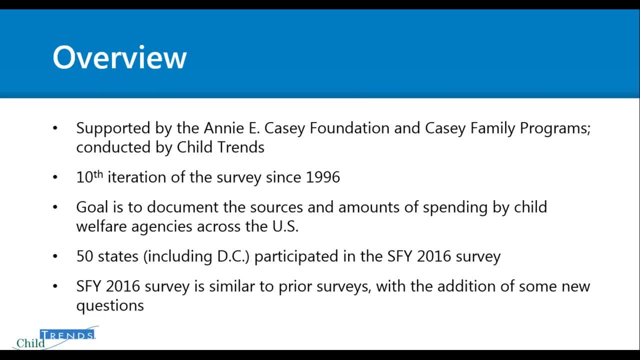 Another thing is that, for those who are familiar with the survey that we conduct, since we do it every other year, this year's survey is very specific. The questions that were asked on the survey were very similar to questions in prior surveys, But we did add several new questions this year. 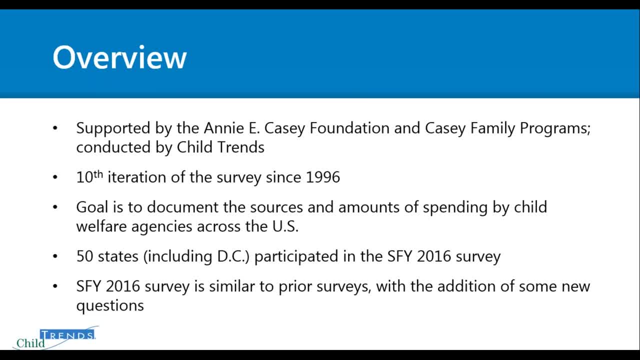 So, for example, we adapt a tool each year to kind of keep up with what's of interest to the field. So, for example, this year we added some questions around prevention services that child welfare agencies fund. We added some questions around spending on family foster care. 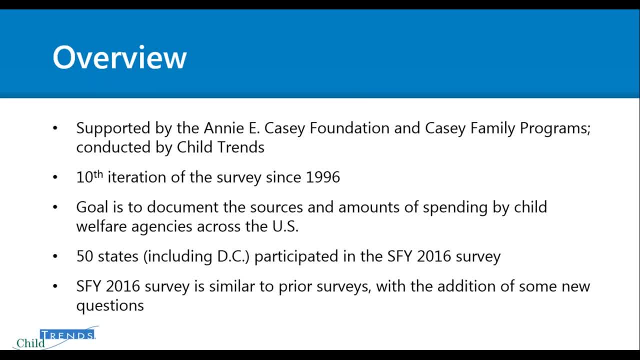 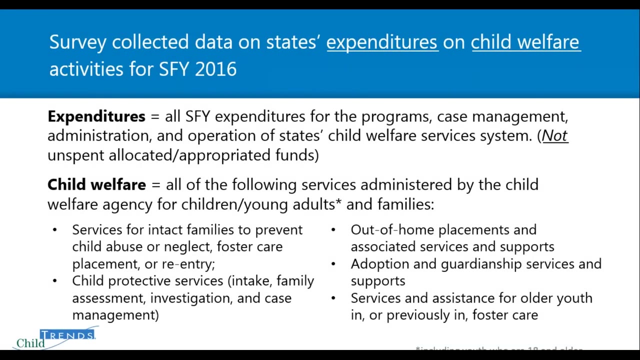 We added some questions around family foster care versus congregate care, So you're not just asking about all out-of-home placements together, but breaking that out a bit more. We asked some questions about spending on evidence-based practices and spending on transportation to maintain school stability and several other new questions, some of which we'll touch on today. 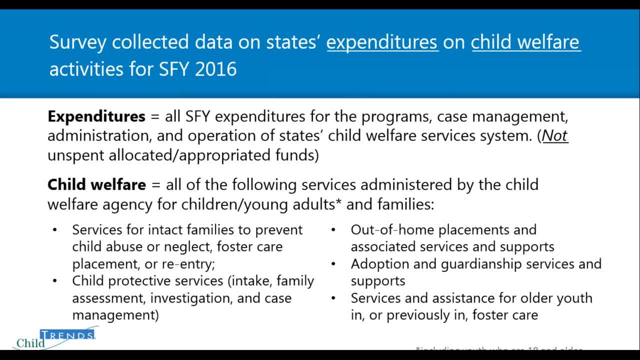 Just a little bit more background before we dive into the findings. The survey collects data on states' expenditures on child welfare activities for state fiscal year 2016.. And by expenditures we mean all state fiscal year expenditures for the programs, case management, administration and operation of a state's child welfare services system. 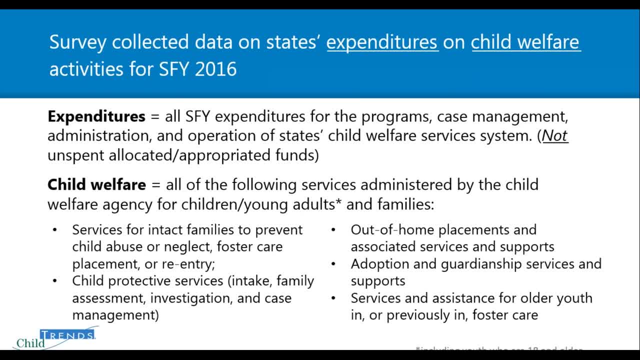 And this is an important distinction from appropriated funds. So we're really focused on the actual expenditures, not any amounts that were appropriated and may not have been spent. for example, And by child welfare we're referring to all of the services and activities you can see here on the screen that are administered by the child welfare agency for children, young adults and families. 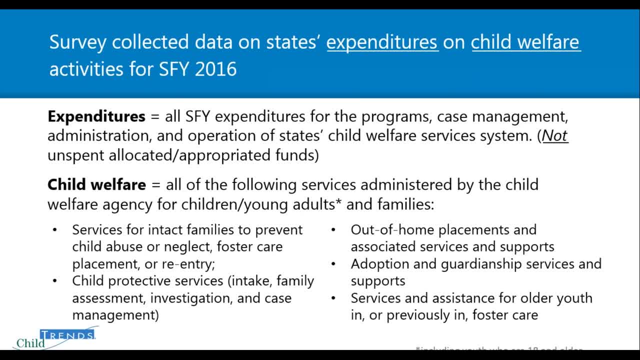 And so this includes services for intact families to prevent child abuse and neglect, foster care, placement or reentry, child protective services, out-of-home placements, adoption and guardianship services, and services and assistance for older youth as well. So, in a nutshell, the survey captures child welfare agency expenditures on child welfare services. 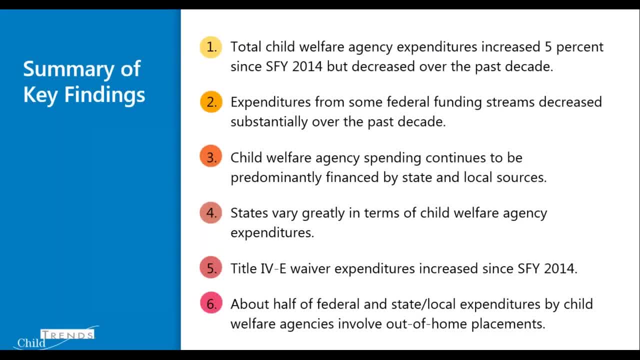 So now I'll hand it over to my colleague, Sarah Catherine, who will provide a quick summary of our main key findings, and then we'll dive into each one. Okay, Thanks, Christina. So again, I'm just going to run through our nine key takeaways and then Christina and I will pass it back and forth to talk about each one of these in more detail. 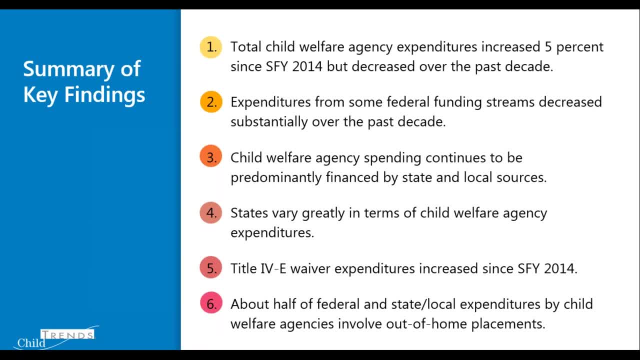 Okay, Thanks, Christina. So again, I'm just going to run through our nine key takeaways and then Christina and I will pass it back and forth to talk about each one of these in more detail. So the first key finding is that total child welfare agency expenditures increased 5% since state fiscal year 2014,. but decreased over the past decade. 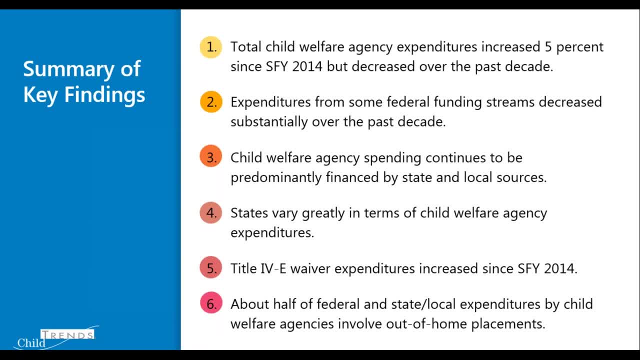 Expenditures from some federal funding streams decreased substantially over the past decade. Child welfare agency spending continues to be predominantly financed by state and local sources. States vary greatly in terms of funding. States vary greatly in terms of child welfare agency expenditures. Title IV-E waiver expenditures increased since state fiscal year 2014,. and for brevity, I will drop the state fiscal year from now on. 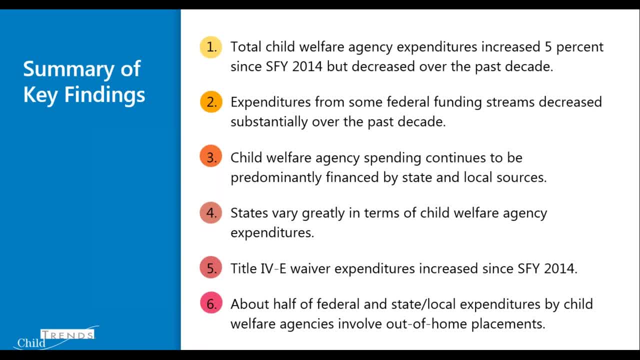 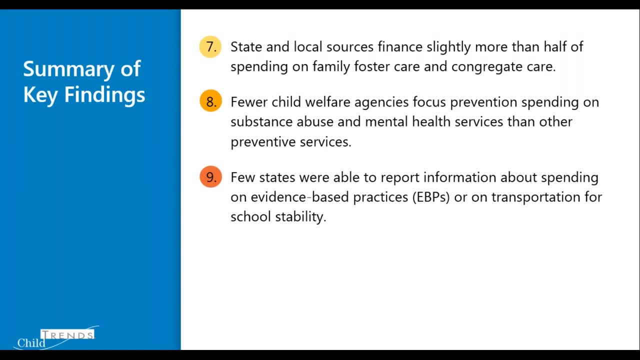 So since 2014, those waiver expenditures have increased. About half of federal and state and local expenditures by child welfare agencies involve out-of-home placement. State and local sources financed slightly more. State and local sources financed slightly more than half of spending on family, foster care and congregate care. 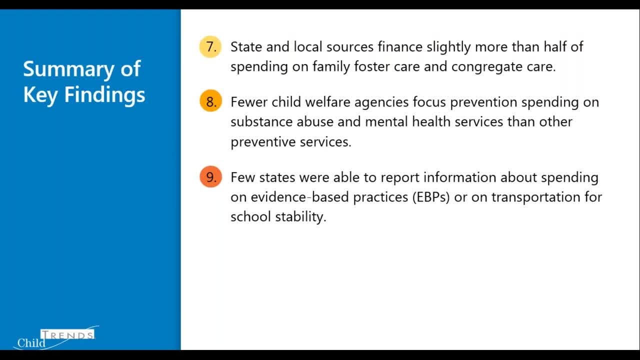 Fewer child welfare agencies focused prevention spending on substance abuse and mental health services than other preventive services. And our last key finding is that few states were able to report information about spending on evidence-based practices or on transportation for school stability. So I'm going to hand it to Christina to start talking about the first finding. 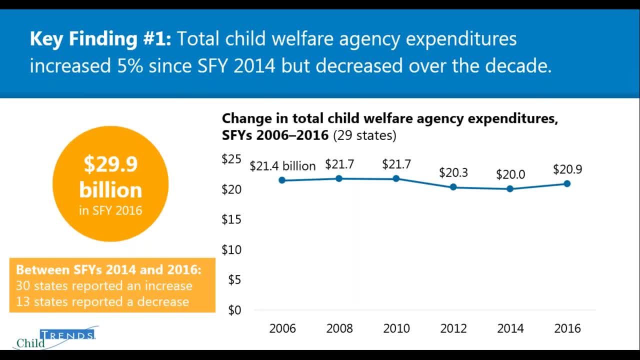 So key finding number one is the total child welfare agency expenditures increased 5% since 2014, but decreased over the decade. So, as you can see here, child welfare agencies reported spending $29.9 billion in federal, state and local funds on child welfare services in 2016.. 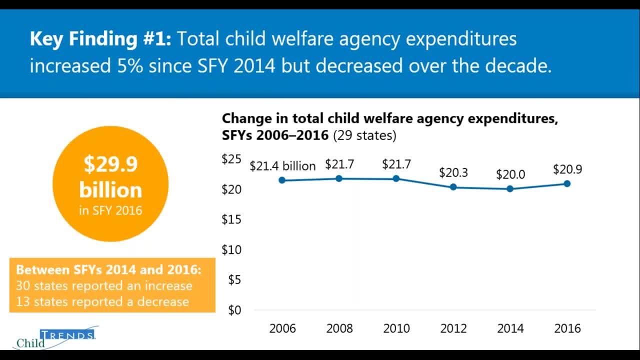 And this represented a 5% increase over 2014.. Among states with comparable data in 2006 and in 2016,. so over the decade, total child welfare agency expenditures have decreased by 1% over that time period And you can see here on this slide the graph shows the trend line over the past decade. 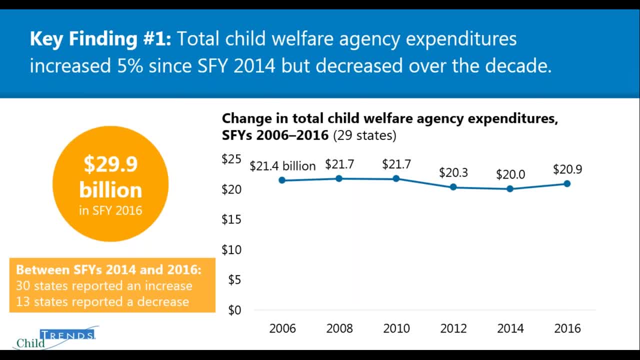 Now, one thing I'll flag here is that the figures presented in the graph reflect an analysis of 29 states, with comparable data across all six years that are reflected in the graph. So you can see here that the figures presented in the graph reflect an analysis of 29 states, with comparable data across all six years that are reflected in the graph. 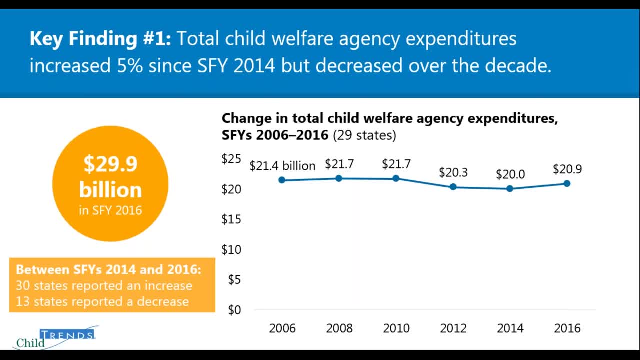 So that's why the 2016 amount in the graph- $20.9 billion- differs from the total reported for 2016,- $29.9 billion, And while that's the overall kind of national picture, there is quite a bit of state variation. 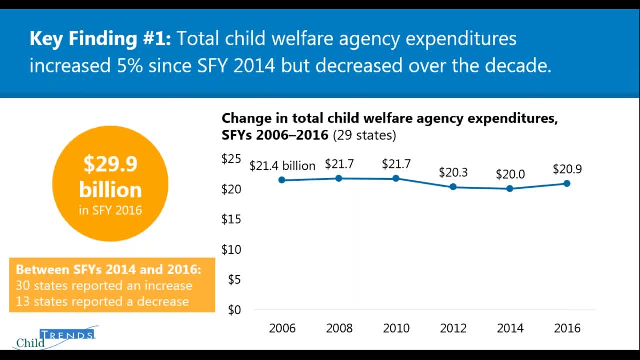 So, despite this overall 5% increase in child welfare agency spending between 2014 and 2016, states varied widely in the magnitude and the direction of changes in their spending. So, despite this overall 5% increase in child welfare agency spending between 2014 and 2016, states varied widely in the magnitude and the direction of changes in their spending. Of the 43 states that had sufficient data in both 2014 and 2016,. 30 of those states reported an increase in total expenditures, while 13 reported a decrease in total expenditures. Of the 43 states that had sufficient data in both 2014 and 2016,, 30 of those states reported an increase in total expenditures, while 13 reported a decrease in total expenditures. Of the 43 states that had sufficient data in both 2014 and 2016,. 30 of those states reported an increase in total expenditures, while 13 reported a decrease in total expenditures. Of the 43 states that had sufficient data in both 2014 and 2016,, 30 of those states reported an increase in total expenditures, while 13 reported a decrease in total expenditures. 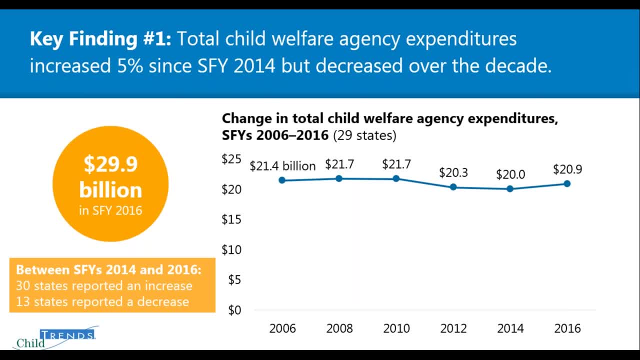 Of the 43 states that had sufficient data in both 2014 and 2016,. 30 of those states reported an increase in total expenditures, while 13 reported a decrease in total expenditures. 30 of those states reported an increase in total expenditures, while 13 reported a decrease. 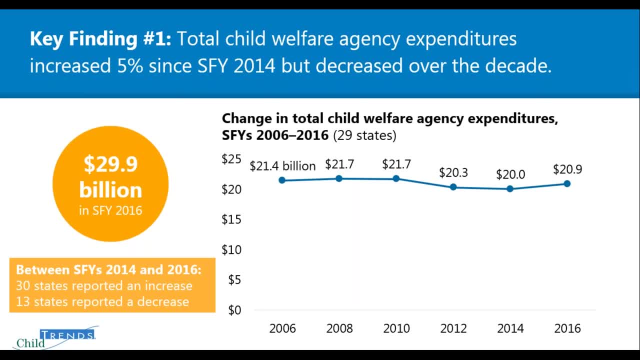 in total expenditures, And these increases ranged from tiny, less than 1% increases to 42% increases in one state, and decreases ranged from a less than 1% decrease to a 25% decrease in one state, And there are many potential explanations for this overall trend that we see at the 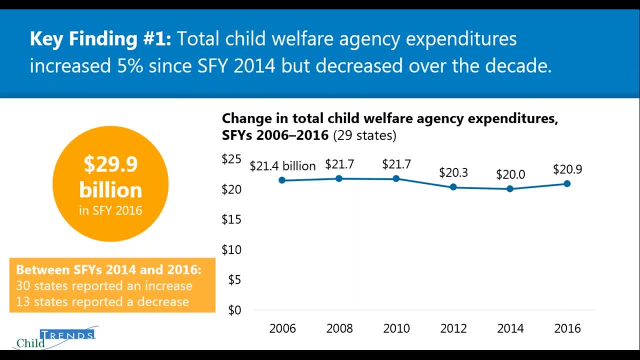 national level. One explanation has to do with changes in the child welfare population. Over the past decade, the number of children in care has decreased by 14%, even though there's been an increase in some more recent years, And this decrease over the decade 2006 to 2016, aligns well with the finding that total 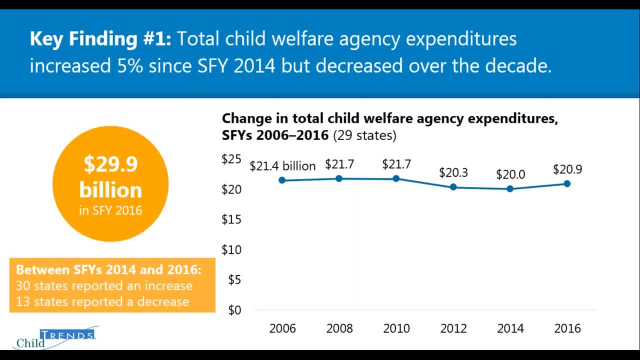 child welfare agency expenditures have decreased, But of course we know the story is often more complex because, beyond serving children in care, child welfare agencies handle referrals for maltreatment, they provide preventive services and do much more, And in fact the maltreatment referral rate has increased over the decade, which does 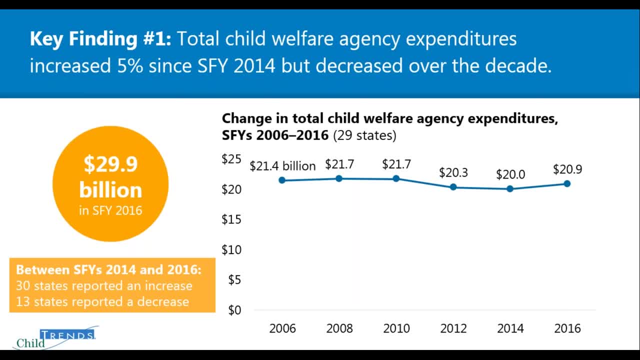 not align with the decrease in spending. Also, the number of children receiving adoption and guardianship assistance, the number of substantiated cases of maltreatment, services and services have all increased. The number of children receiving adoption is also decreasing And the numbers of children receiving adoption have increased. 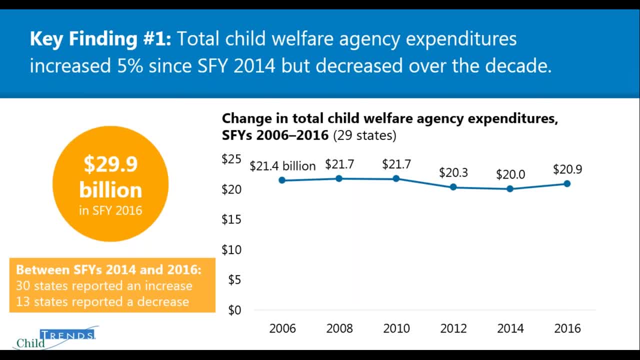 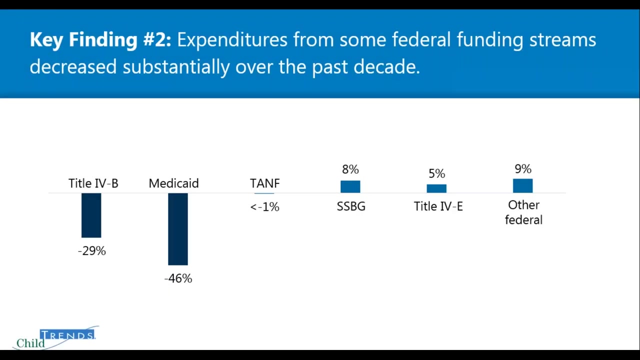 So, while the number of children receiving adoption may impact expenditures, it's not the only explanation. Other explanations relate to how expenditures of particular funding streams have changed over time, which we'll show on the next slide, And this is a good example of how the number of children receiving adoption has changed. 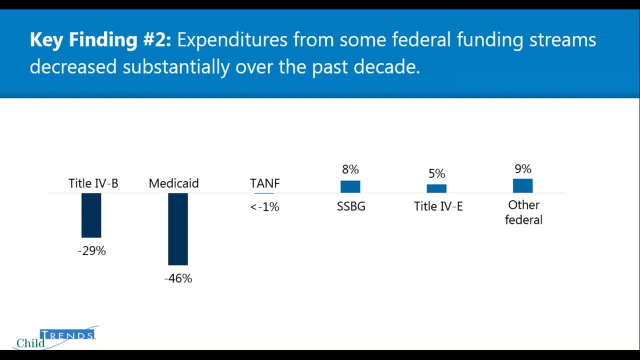 So let's talk about the numbers. Let's talk about the numbers. This is a graph. key finding number two, which is expenditures from some federal funding streams decreased substantially over the past decade. and before we get into the trends here, I'll first provide a brief overview of these funding streams. first, 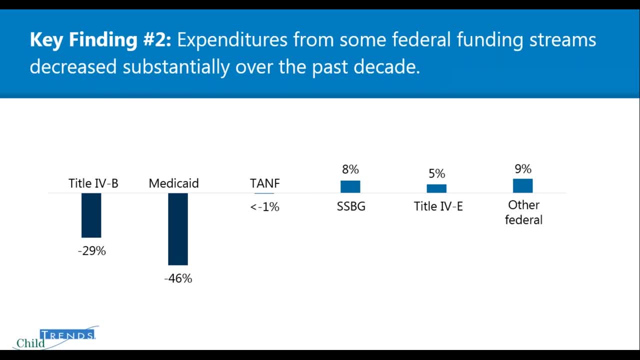 listed here is title 4b of the Social Security Act, which is a funding source that's specific to child welfare, and it can be used for the prevention of maltreatment, family preservation, family reunification, services for foster and adopted children, training for child welfare professionals and adoption. 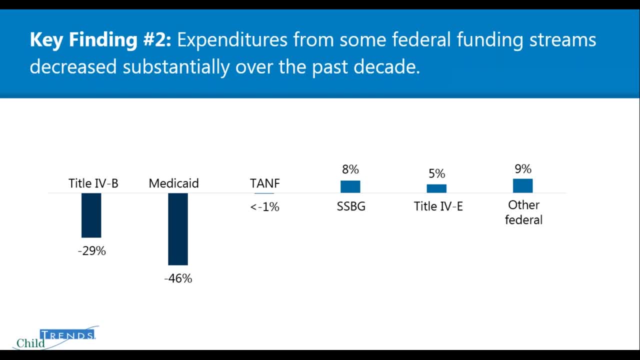 promotion activities. there's also Medicaid, which provides health coverage and services, including clinical behavioral health services, to low-income individuals. one thing to keep in mind about Medicaid is that, on our survey, states only report Medicaid dollars that cover costs borne by the child welfare agency or for which the child welfare agency pays a non-federal 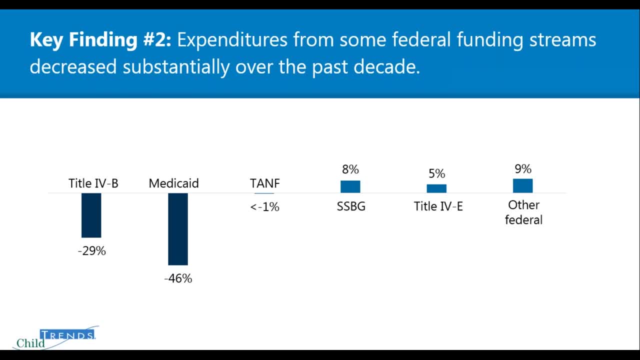 match excludes Medicaid funded costs for the child welfare population that were born by other agencies like health departments, so that means it excludes costs associated with health care coverage. there's also temporary assistance for needy families, or TANF, which addresses for overarching purposes which are defined in statutes as providing assistance to needy families. 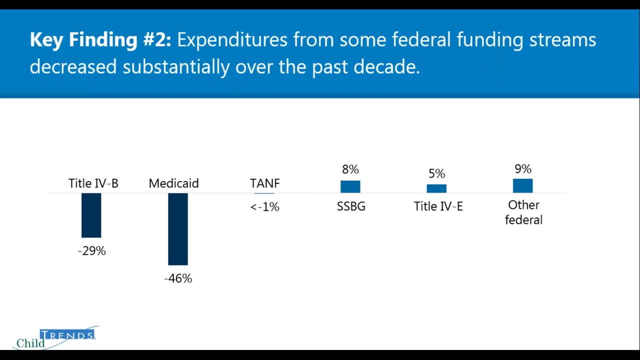 so that children may be cared for in their own homes or in the homes of relatives. TANF also seeks to end the dependence of needy parents on child welfare services. TANF provides some government benefits by promoting job preparation, work and marriage. it seeks to prevent and reduce the incidence of out of wedlock. 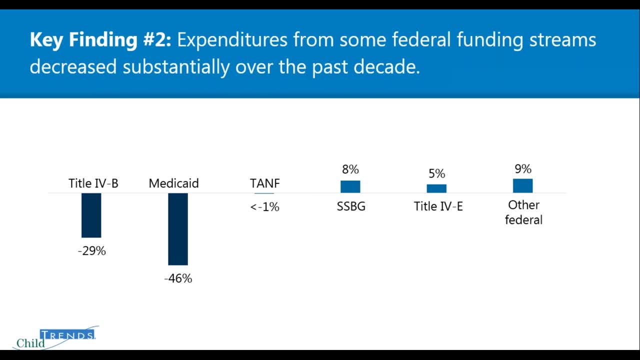 pregnancies and encourage the formation and maintenance of two parent families. and while TANF is primarily thought of as a cash assistance program for low-income families, only around a quarter of TANF dollars spent in federal fiscal year 2016 were used to provide basic cash assistance for. 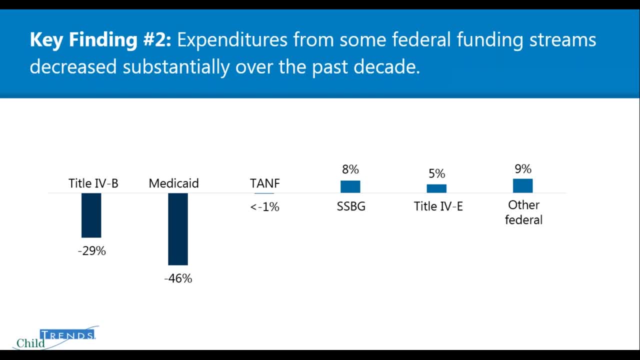 families, and because TANF funds are designed to flexible, they can be used for a wide array of services and supports aimed at achieving one of the program's four goals, And so states use this flexible funding for supporting child welfare activities. There's also the Social 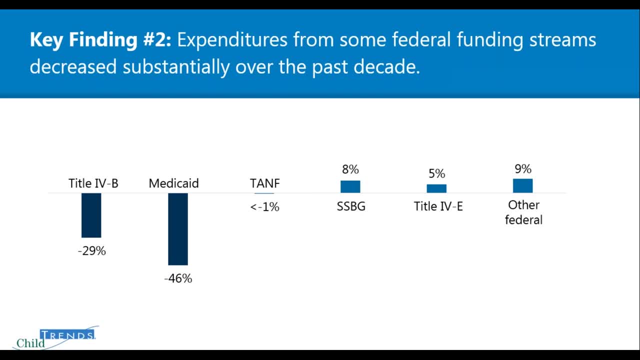 Services Block Grant SSBG, which is a source of flexible funding to promote self-sufficiency, prevent or remedy child maltreatment, reduce inappropriate use of institutional care and more, And SSBG can be used for a wide variety of purposes. 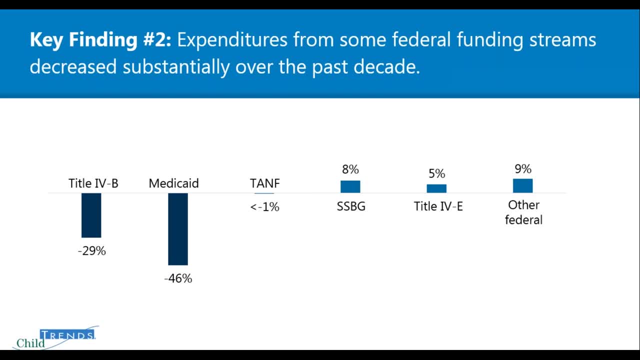 with child welfare being one of them. And then Title IV-E of the Social Security Act is another funding source specific to child welfare and can be used for foster care, adoption, guardianship, transition supports for eligible children and child welfare workforce training. And Title IV-E is the 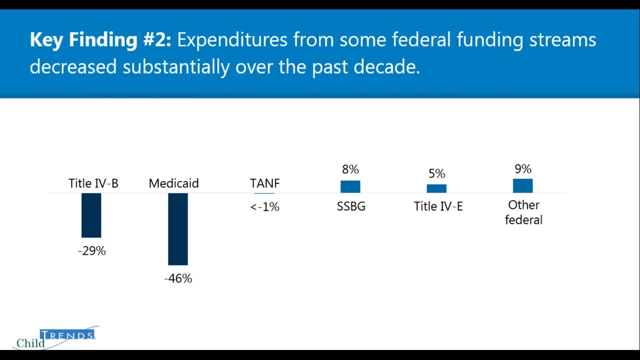 largest federal funding stream for child welfare agencies. And then, finally, states may use other federal funding streams to fund child welfare services, such as the Child Abuse Prevention and Treatment Act, CAPTA, Adoption and Guardianship, Acquisitive Awards, and more So. with that overview, as you can see on, 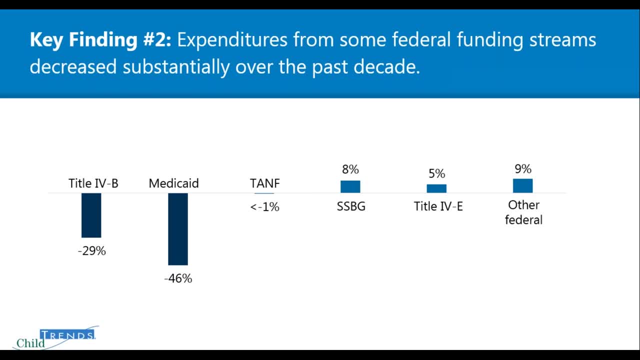 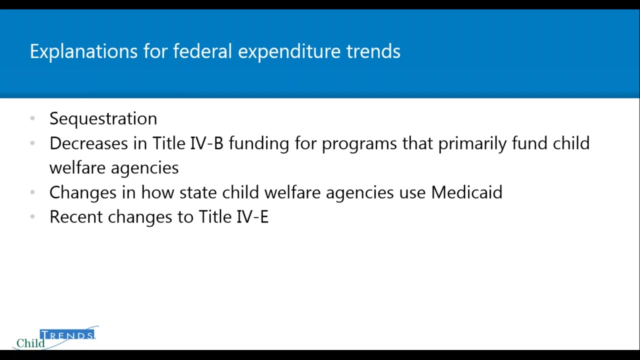 this slide. Title: IV-B and Medicaid child welfare agency expenditures decreased quite substantially over the past decade, But on the flip side, expenditures of other federal funding sources experience increases, like a 5% increase in IV-E since 2006.. So what's behind these trends? One explanation behind these federal expenditure. 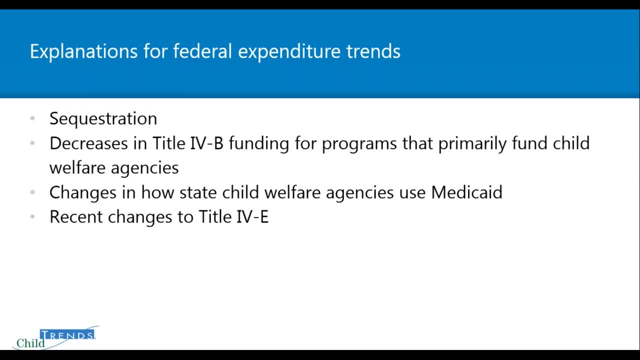 trends is sequestration. The Budget Control Act of 2011 stipulated automatic spending cuts starting in federal fiscal year 2013,. if Congress was unable to reduce spending on its own, Most child welfare funding sources were not affected. sequestration, but two sources, 4B and SSBG, were affected, And the effects of 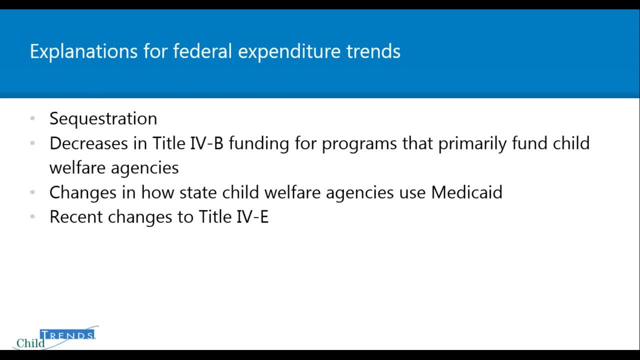 sequestration are likely reflected in, but do not account for, all of the 29% reduction in 4B spending over the past decade. However, you know, in shifting to SSBG we saw that SSBG spending by child welfare agencies increased by 8% since. 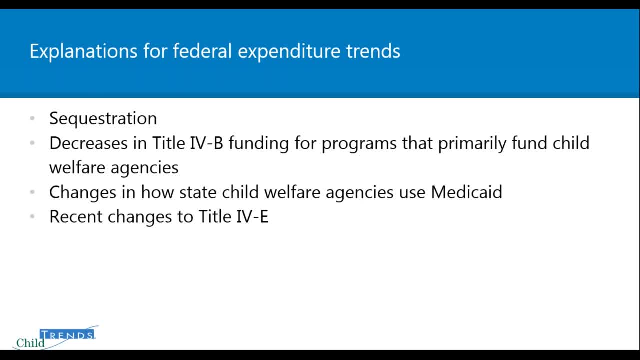 2006.. So at first glance this may seem counterintuitive, given sequestration, but SSBG is not solely dedicated to child welfare. In fact, the total state SSBG spending on services most relevant to child welfare agencies has increased in. 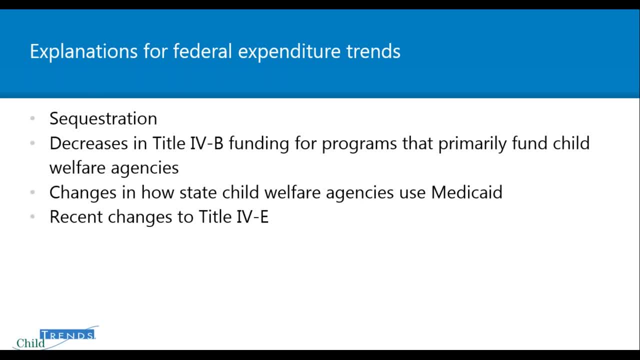 recent years, while spending on services less relevant to child welfare agencies, like services and supports for vulnerable and elderly adults, has decreased. So, in other words, while the total SSBG allocation provided to states has shrunk due to sequestration, it appears that child welfare agencies are accessing a 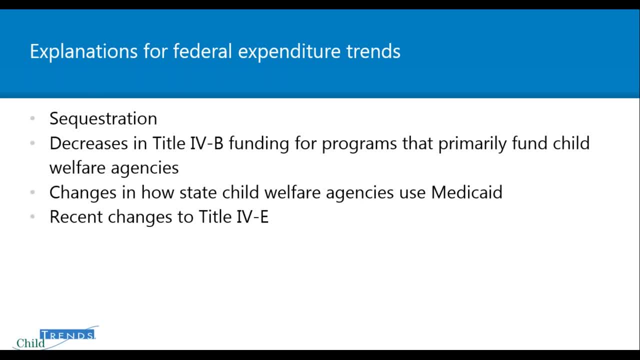 greater proportion of these allocations than in the past, And there's also decreases in 4B funding for programs that primarily fund child welfare agencies. I should say So: apart from sequestration, appropriations for 4B, programs that primarily fund child welfare agencies have decreased over the past decade. 4B is made up of: 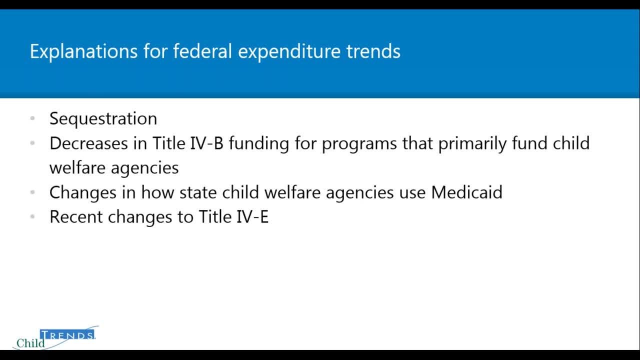 two subparts, and subpart two is called the Promoting Safe and Stable Families Program, or PSSF, And that program primarily funds family support, family preservation, reunification and adoption promotion and support activities. And out of that total appropriation for the PSF program, funds must be set aside for 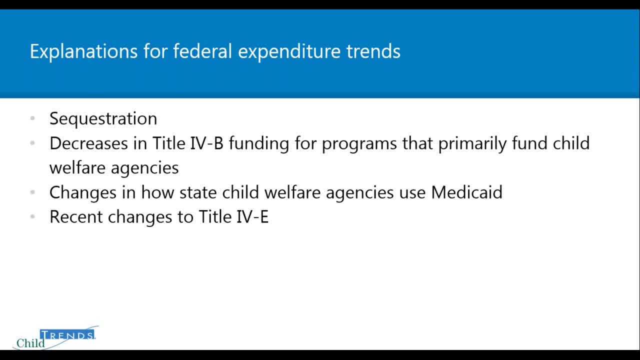 certain things, one being the Court Improvement Program. Another example is regional partnership grants that seek to improve outcomes for children affected by parental substance abuse. There's also a set-aside for improvements to caseworker visits and research, evaluation, training and technical 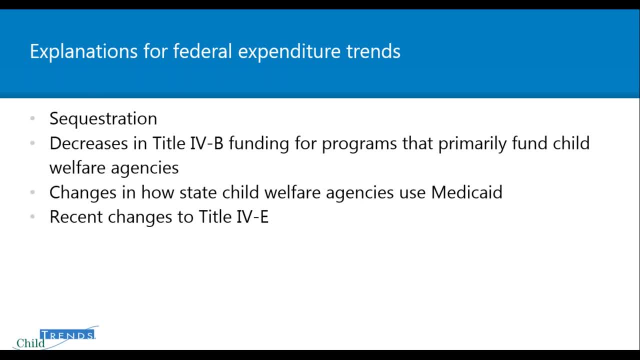 assistance. So after those set-asides are funded then the remaining PSSF dollars under 4b are available to child welfare agencies for services. so in federal fiscal years 2006 to 2010, part of the total cost of the court improvement. 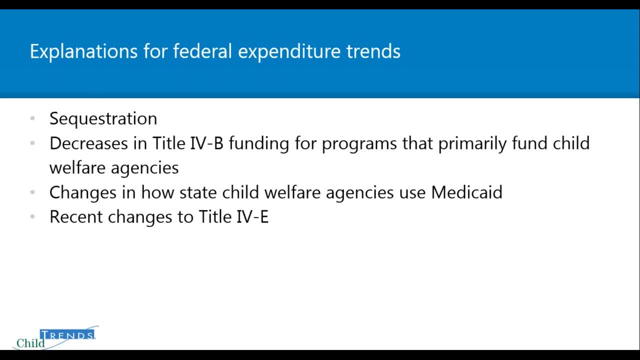 program was funded outside of title 4b, but then, starting in 2011, the full cost began to be covered under the PSSF program and, since court improvement dollars go to courts and not child welfare agencies, this means that, over the course of the past decade, fewer 4b dollars were left over for child welfare. 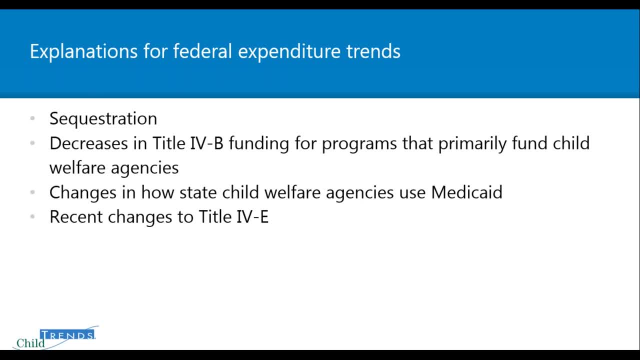 agencies after the court improvement program set aside and likewise the regional partnership grants started in fiscal year 2007. since many RPG grant he is are not child welfare agencies, the addition of the RPG set aside also reduce the amount of PSSF dollars available to shovel for agencies and the 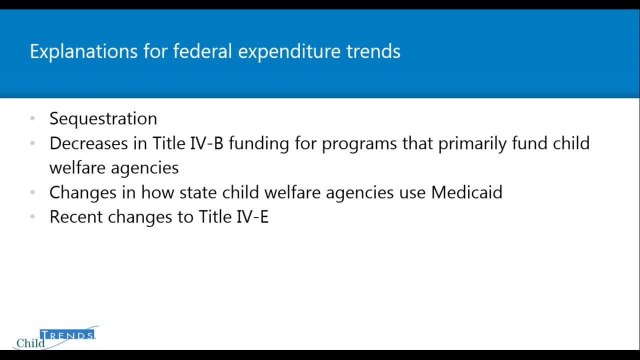 Appropriation for the one PSS, SSF set-aside debt that is directed to child welfare agencies, funds to improve paid-to-worker visits. that one actually declined over the decade, So that helps explain why Title IV-B expenditures have gone down. There are also changes in how 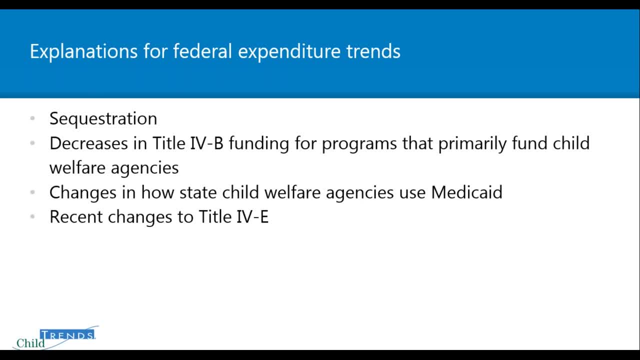 state child welfare agencies use Medicaid. The observed decrease in child welfare agency Medicaid expenditures over the decades may be due to changes in how state child welfare agencies use Medicaid, rather than a decrease in Medicaid services for this population. In fact, between 2006 and 2016,. fewer states 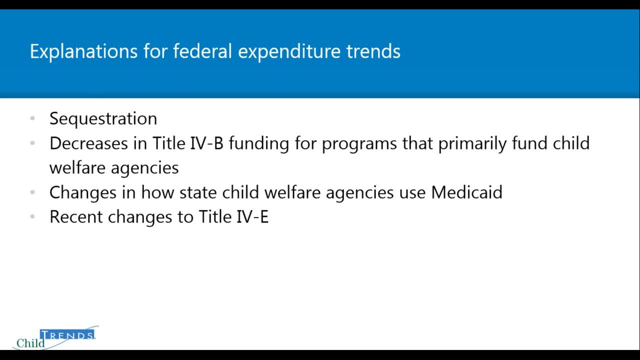 reported that the child welfare agency accessed Medicaid dollars. So, for instance, child welfare agencies in some states reported that they have shifted costs for Medicaid-funded services to another agency, bundled or unbundled services and transition between fee-for-service and Medicaid-funded services. So, for example, 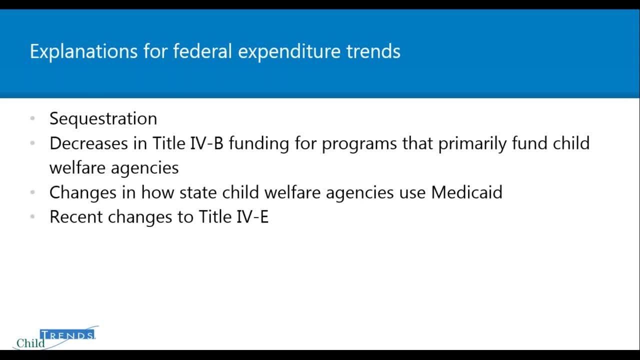 a large number of states actually did access Medicaid dollars for Medicaid services other than for child welfare contracts and skill loans and service services in managed care systems, And these are administrative changes that can affect how Medicaid is accessed in each state and could contribute to the 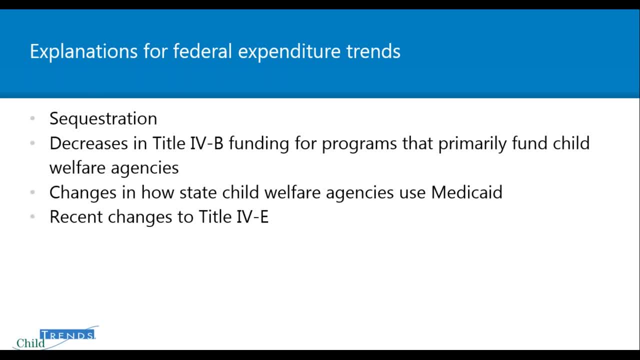 observed decrease in child welfare agency Medicaid expenditures, But without surveying how all entities in a state access Medicaid dollars for the child or whether Medicaid funded services are more or less available to the child welfare population. However, a 2014 analysis conducted by the Congressional Research Service 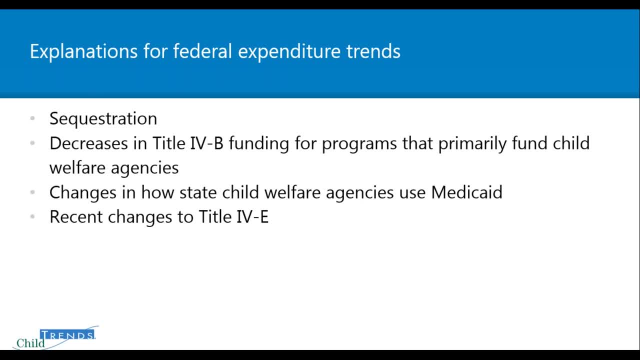 that looked at total Medicaid spending on a subpopulation of children involved with the child welfare system showed that total Medicaid spending on this population did not change significantly between federal fiscal years 2005 and 2010.. However, this report did show that total Medicaid spending on this population for rehabilitative services 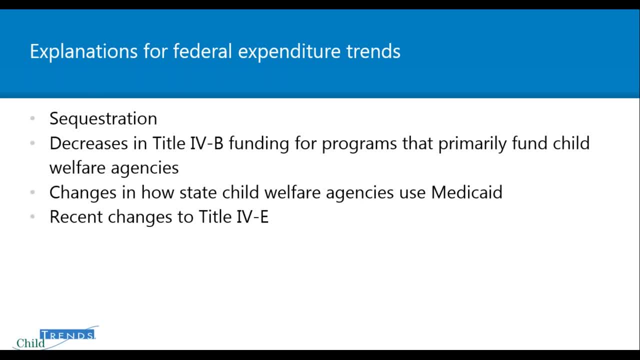 and targeted case management decreased between 2005 and 2010.. And these are types of Medicaid services that child welfare agencies tend to use Medicaid for. Therefore, while total Medicaid spending on this population remained relatively stable, based on the CRS report, the kinds of services being used changed. 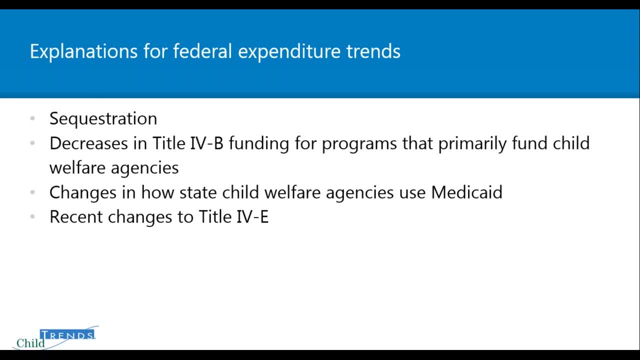 which could help explain why child welfare agency Medicaid expenditures went down. And then, finally, there have been recent changes to Title IV-E And, as we showed on the prior slide, Title IV-E expenditures increased by 5% over the decade, And this is because states are communicating with each other. 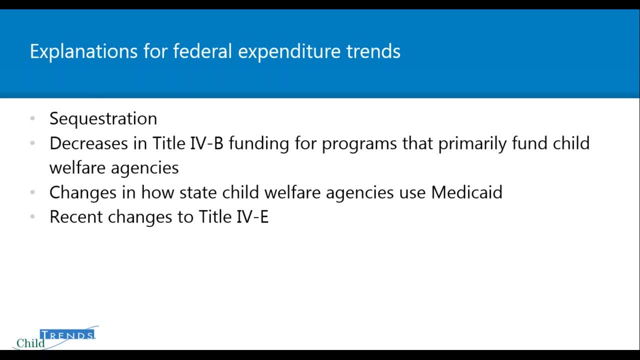 We're continuing to see the impact of the Fostering Connections Act of 2008,, which influenced expenditures in several IV-E programs. For example, this legislation broadened the adoption assistance eligibility criteria, resulting in an increase in the number of children receiving adoption subsidies. 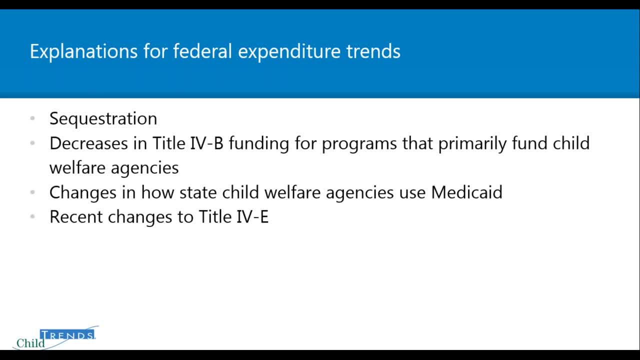 and the overall funding level of the adoption assistance program. Likewise, there's been a 45% increase in IV-E guardianship assistance program expenditures between 2014 and 2016.. This is because more states have taken up the option made available in the legislation. 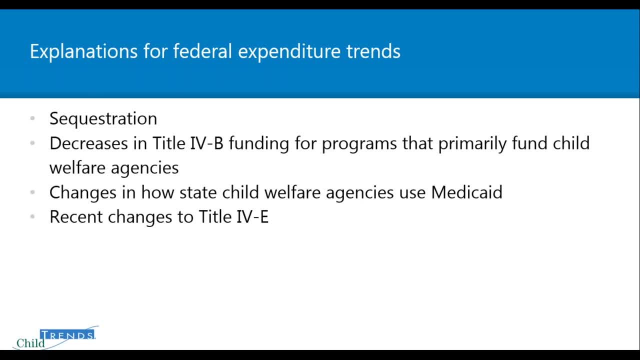 that allows for IV-E reimbursement of assistance payments made to eligible relative caregivers who opt to pursue legal guardianship. In addition, most states that already had a IV-E guardianship assistance program saw that program expand in 2016.. In addition, the Fostering Connections Act allowed states to claim additional 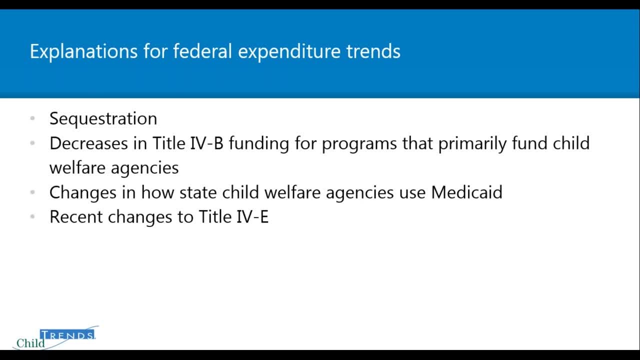 training costs starting in 2009, and allowed for IV-E to be used for the costs for youths ages 18 to 21 who remain in foster care, contingent on other requirements, And then beyond Fostering Connections, the increase in total IV-E expenditures. 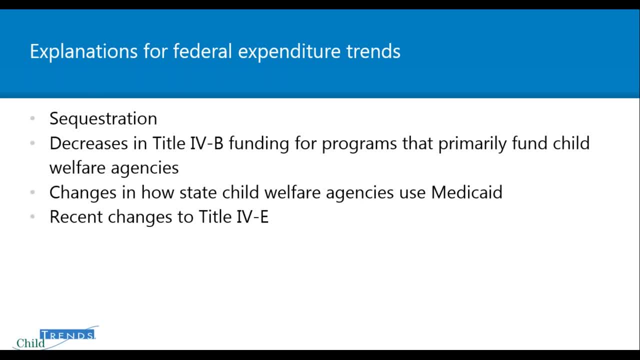 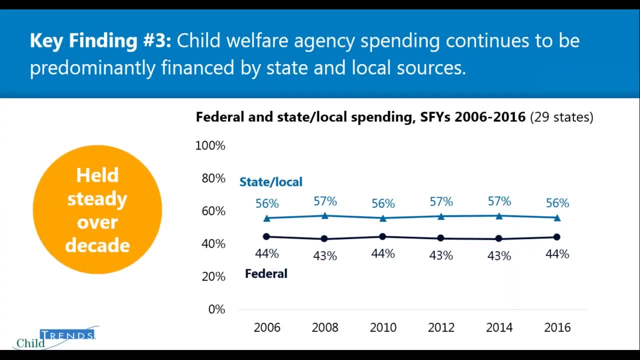 was also driven by an 82% increase in Title IV-E waiver expenditures between 2014 and 2016,, which we'll talk about a little bit later. All right, so I'm going to move on to our third key finding, which is that child welfare agency spending continues to be predominantly financed. 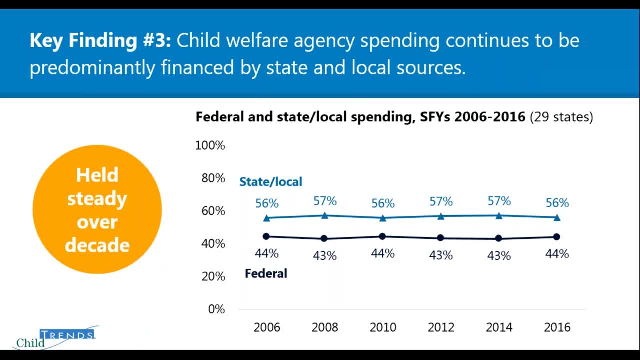 by state and local sources. In addition to federal sources, states spend their own dollars on child welfare services and activities. State and local funds are used to match federal funds or to meet required maintenance of effort for a federal program and to pay for additional costs that the federal funds do not cover. 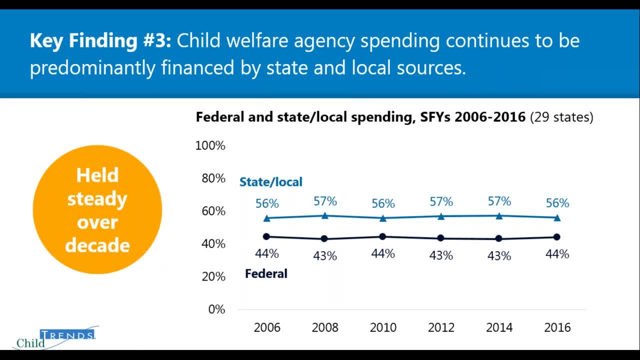 For most states, these funds come primarily from state dollars, though some states report using more local dollars than state dollars. In 2016,, 56% of all dollars spent by child welfare agencies came from state and local, as opposed to federal, sources. 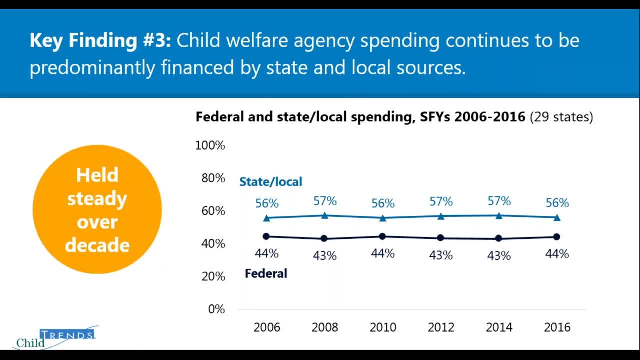 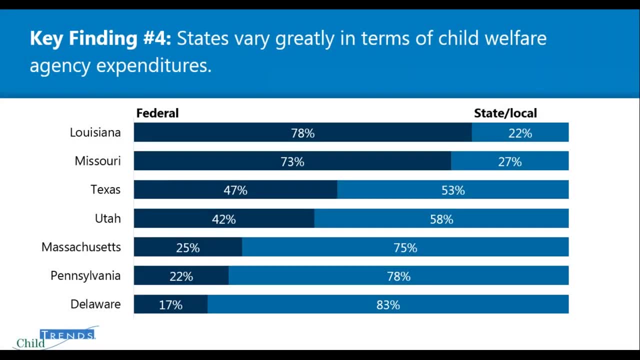 And, as you can see here on this graph, during the past decade these proportions have held steady. Key finding number four, and this isn't surprising- is that states vary greatly in terms of child welfare agencies' expenditures. The graph here gives you some examples of how states vary. 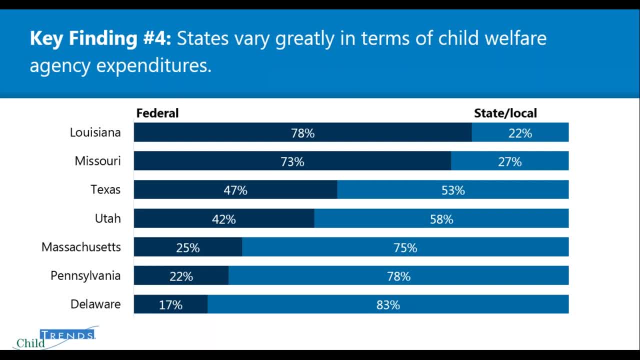 in the proportion of funds that come from federal versus state and local sources, And these are just some example states that we pulled to show variation and the breakdown for all states is available in our main report And, as you can see here, Louisiana had the largest number. 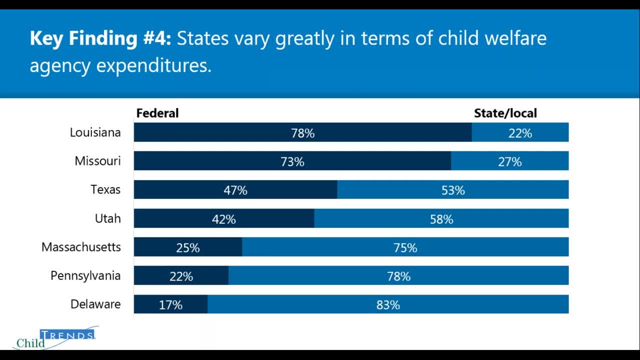 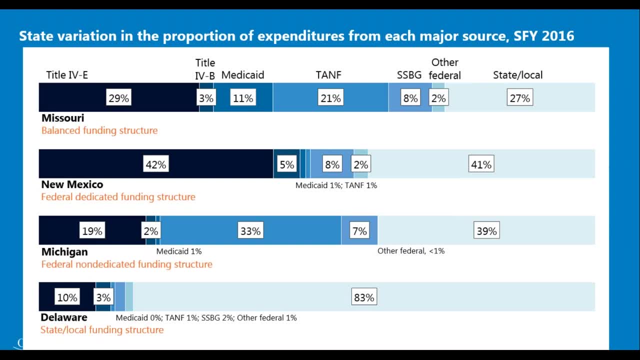 and the largest proportion of funds from federal sources at 78%, and then Delaware had the smallest proportion, at 17%. And now we're going to break the previous slide down a little bit further. This slide shows the breakdown of all sources for a select few states. 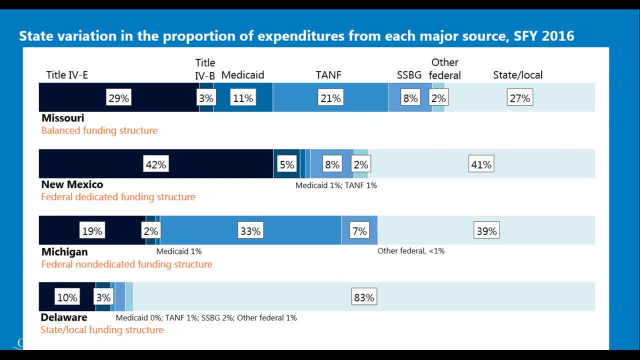 So states not only vary in terms of how they use their federal versus state and local dollars, but they also vary regarding their use of federal sources. So we've identified four different types of funding profiles and we've shown you one example of each here on this slide. 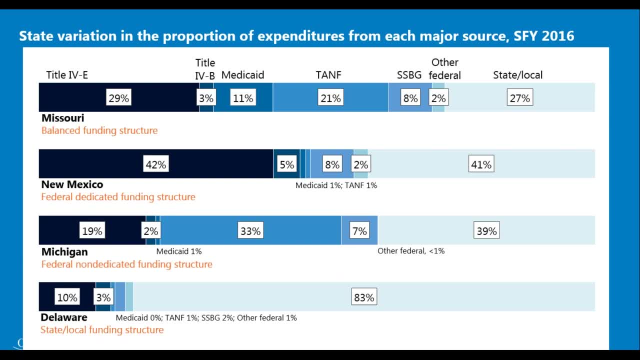 The first one is balanced funding structure, in which the child welfare agency uses a mix of federal and state and local funds and draws on a diversified selection of federal funding sources, both those that are dedicated to funding child welfare services as well as others. The next one is a federal dedicated funding structure. 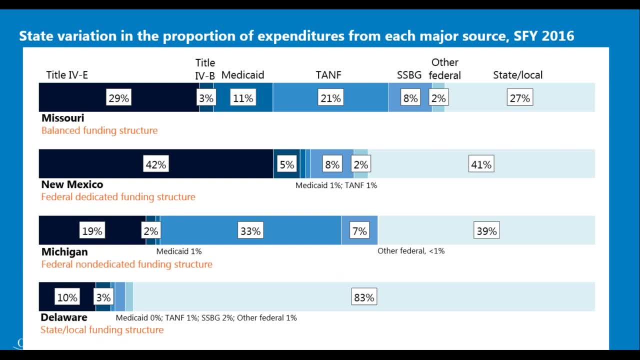 in which the child welfare agency uses more federal than state and local funds and draws primarily from dedicated federal funding streams. When I say dedicated, I mean sources that are dedicated specifically to funding child welfare services, like Title IV-E and Title IV-B. The third one is our federal non-dedicated funding structures. 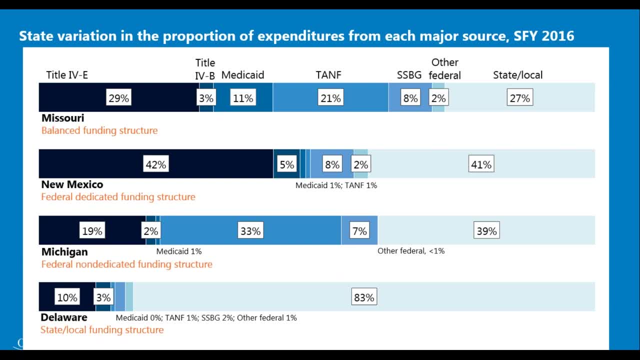 in which, again, the agency uses more federal than state and local funds, but relies heavily on non-dedicated funding streams, And by non-dedicated we mean sources that can also be used by a variety of agencies to fund other types of services. 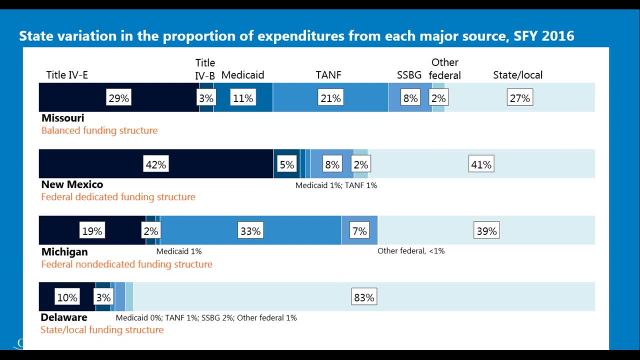 So these would be like Medicaid, TANF or SSPT, And the last one is a state and local funding structure in which the child welfare agency relies primarily on state and local funds instead of federal sources. So I'm sure a big question that a lot of you have is: 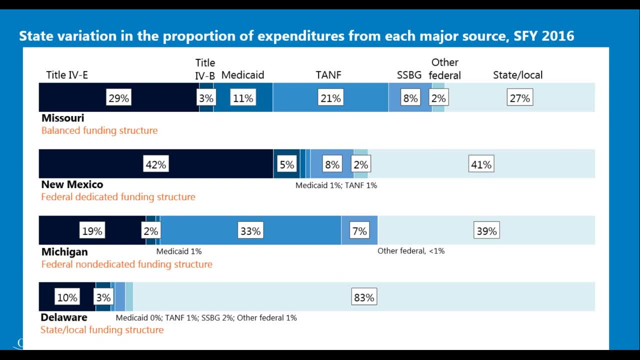 well, why do they vary so much? We've identified a few factors, including the ability to meet match requirements, While most states want to maximize the use of open entitlement funds such as IV-E, which allow for federal reimbursement without a set ceiling. 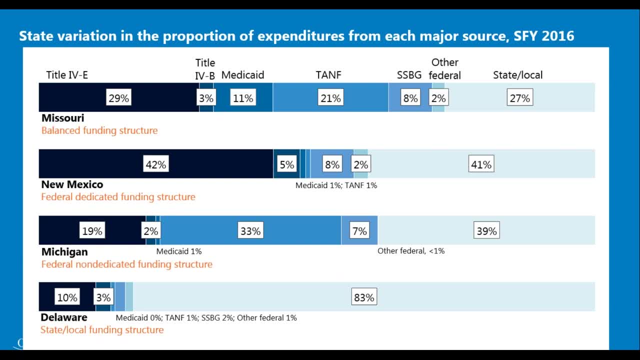 they have to have sufficient funds to meet the match requirement. So, for example, Title IV-E has a 50% match requirement for administrative costs. Therefore, the availability of state and local dollars limits the use of some federal funding sources, For instance if a state has limited state and local funds. 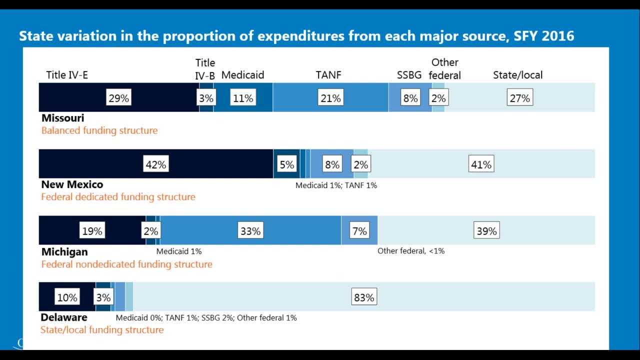 it may prefer to rely more heavily on federal funding streams and do not require it to contribute state and local matching funds like SSPT. The characteristics of children served by the child welfare agency can also affect which funding streams are used, and that's due to eligibility criteria associated. 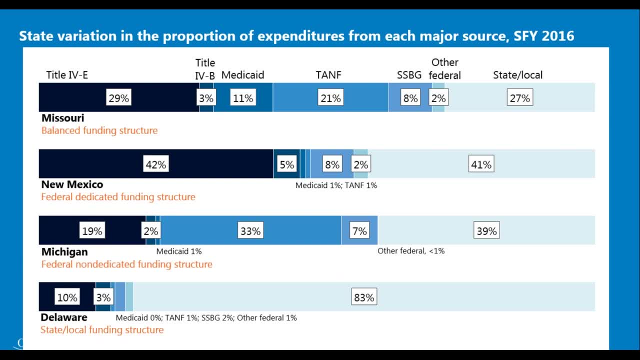 with certain funding sources. For example, Title IV-E has an income eligibility requirement. that means that only certain children are eligible for IV-E reimbursement, For instance, if a state has, you know, only a few eligible children that are eligible for Title IV-E or Medicaid. 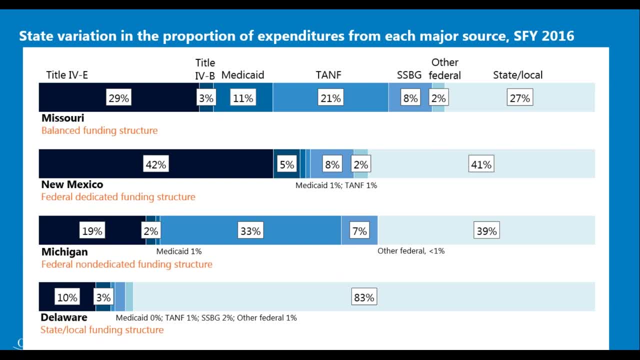 the child welfare agency is going to be limited in its Title IV-E and Medicaid expenditures. There's also competition from other agencies, such as TANF agencies, for non-dedicated funding streams, And this means that some child welfare agencies may find it difficult to access those sources. 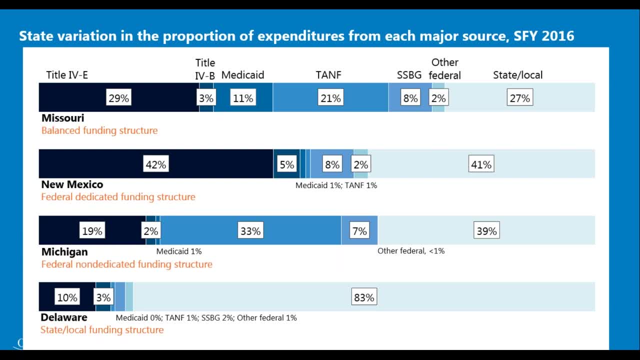 And this competition can be particularly great in times of crisis economic downturns, when pressures on TANF cash assistance are higher and leave fewer dollars available for other purposes, And in those cases, a child welfare agency may rely more heavily on funding streams that are dedicated. 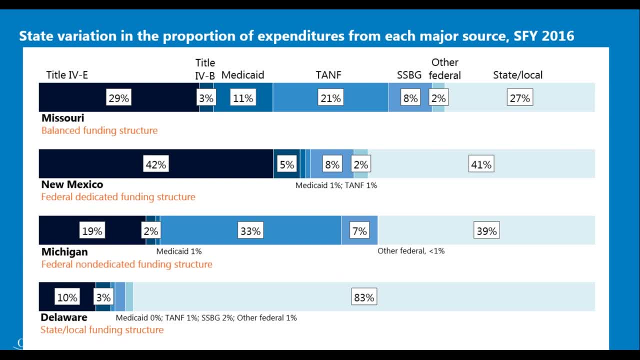 to child welfare purposes than other, more broader funding sources. And the last factor we identified are federal funding stream requirements. Some federal funding streams have requirements, such as eligibility determination, that can place a high administrative burden on states, which can be costly and can outweigh the benefit of receiving the funding. 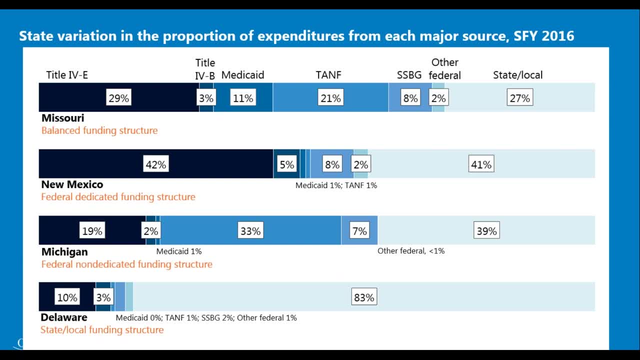 And this could cause some states to rely more heavily on state and local funds. And you know, like I said, we showed you one example of each one of these funding structures here, but in the appendices of our report you can find this funding breakdown for every state. 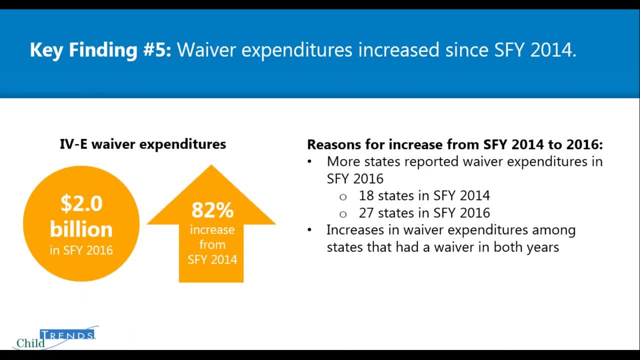 Great. So key finding number five is that Title IV-E waiver expenditures increased since 2014.. Before we dig into this, first a little bit of background about waivers. The federal government can waive state compliance with specific Title IV-E eligibility requirements for states participating in what are called waiver projects. 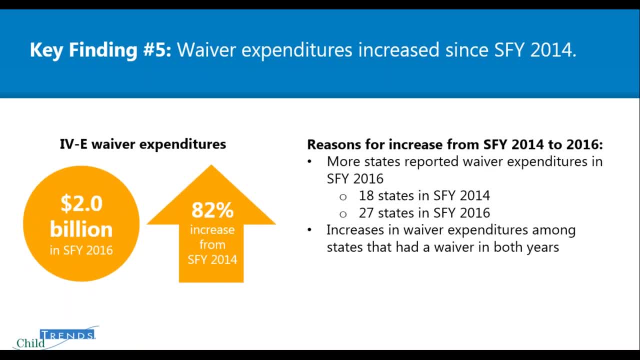 For example, for a child to be eligible for the Title IV-E foster care program, they must meet eligibility criteria related to things like income, circumstances around their entry into care and the type of placement that they're in, And there are also requirements around the types of services. 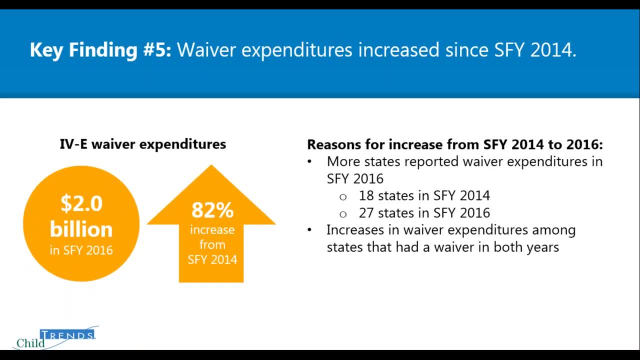 and supports that can be reimbursed by IV-E. And if a state has a IV-E waiver, the federal government can waive those specific IV-E requirements and the state can use IV-E funds to cover services for children who are not traditionally eligible under IV-E. 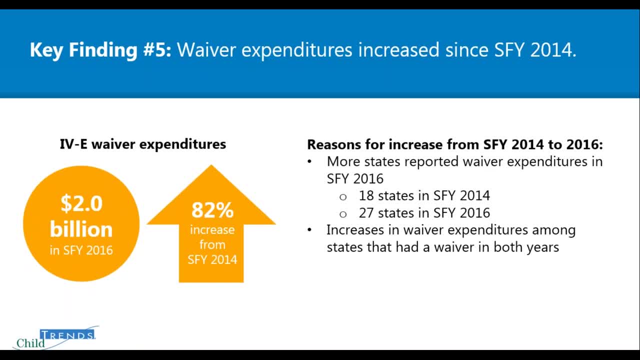 and pay for services that aren't typically IV-E reimbursable. So the waiver projects are designed to promote innovation in the design and delivery of child welfare services, to support child safety, permanency and well-being, And, while states vary in terms of the goals, 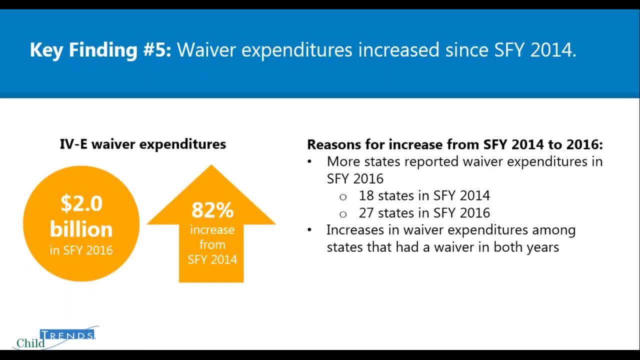 of their waiver projects, many focus on preventing abuse or neglect, reducing the occurrence of reentry into foster care and supporting permanency. So of the total $29.9 billion in reported child welfare agency expenditures for 2016,, about $2 billion of that is associated. 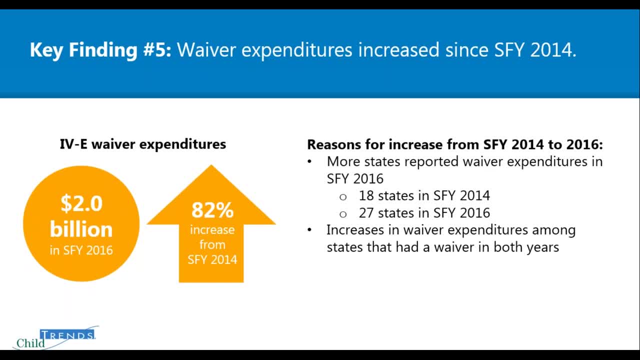 with federal IV-E waiver-related expenditures And between 2014 and 2016,. those waiver expenditures have increased by 82%, like I mentioned a couple of minutes ago, And this increase was due to more states reporting waiver expenditures in 2016.. 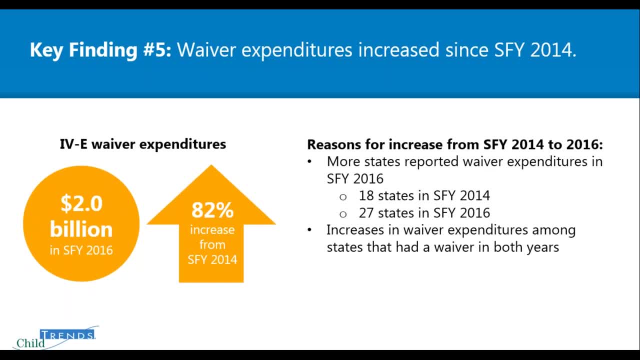 Specifically, 18 states reported waiver expenditures in 2014, compared to 27 states in 2016.. But this increase is also due to increases in waiver expenditures among states that had a waiver in both years. So, for instance, New York's waiver spending. 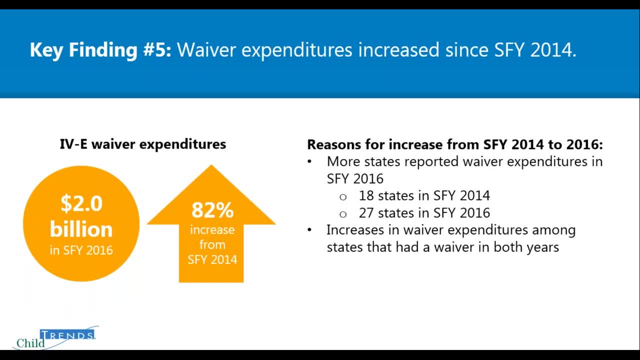 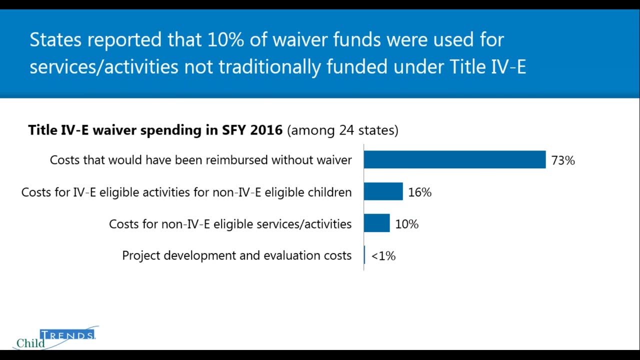 increased by almost 600% And in fact, the majority- around three-quarters or so- of the increase in waiver spending was due to existing waiver states expending more waiver dollars, And funds accessed through a waiver can be used to cover four different types of expenditures. 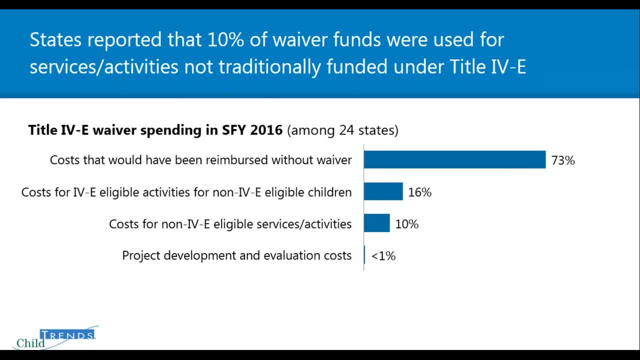 One are costs that would have been reimbursed without the waiver. These are the costs for those IV-E eligible children to receive IV-E eligible activities. There's also costs for IV-E eligible activities for children who would not qualify for IV-E under traditional eligibility criteria. 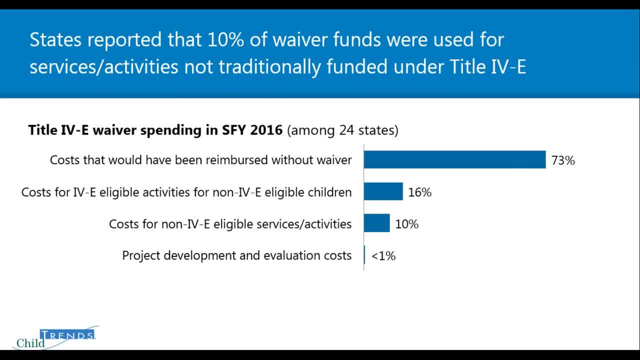 And then, third, there's costs for activities that fall completely outside of traditional IV-E eligible categories for any child, regardless of their eligibility. And then, finally, there are project development and evaluation costs that are mandated by participation in the waiver, And states reported that in 2016,. 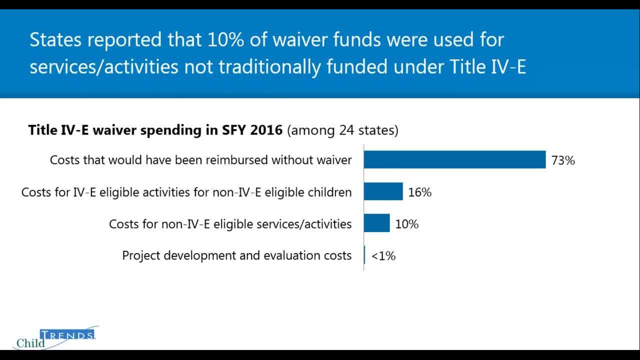 10% of waiver funds were used for services and activities not previously reimbursable under IV-E, And states reported paying for activities like in-home services or prevention services and evidence-based practices. And the remaining 89% of the waiver funds were spent on activities. 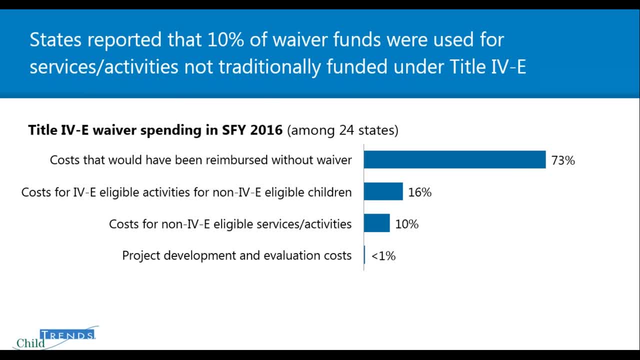 like maintenance payments and caseworker activities on behalf of children in care that would have been permitted without the waiver. However, states spent 16% of total waiver expenditures on activities for children who, without the waiver, would not have been eligible for IV-E due to income placement type. 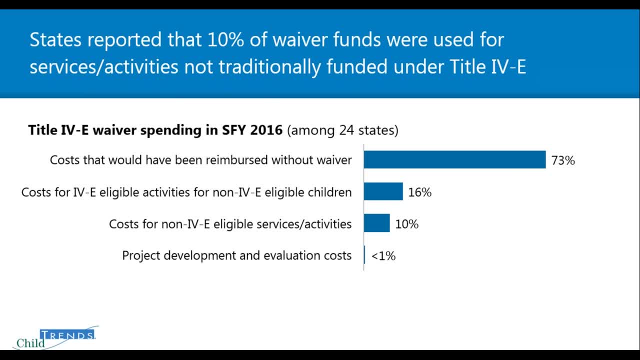 or their circumstances related to their entry into care. So, with the waivers currently set to expire later this year, states will have to find other funds to cover those services and activities And if 2016 expenditures are indicative of waiver spending in more recent years, 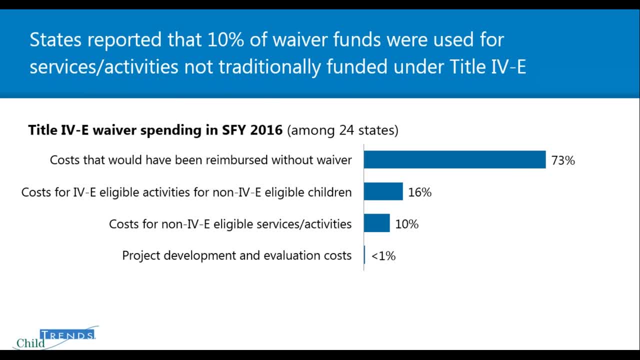 then the end of the waivers would result in a loss of more than $300 million in Title IV-E funds, which is calculated as 26% of the total waiver expenditures reported by these 24 states that could break out their waiver spending. A few things to keep in mind is that states with waivers 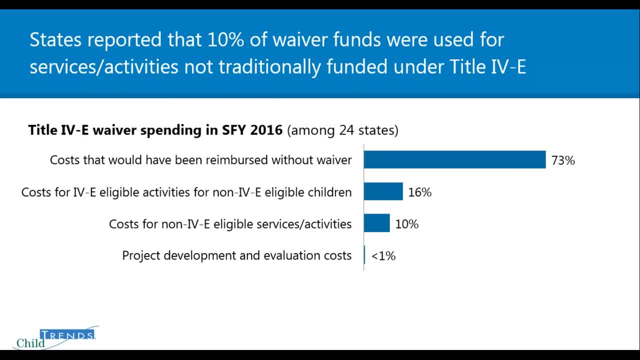 must still provide traditionally eligible services like foster care, So they're limited in how much of their waiver dollars can go to new, innovative services. And also, while not asked on the Child Welfare Financing Survey, states could be using non-IV-E funds. 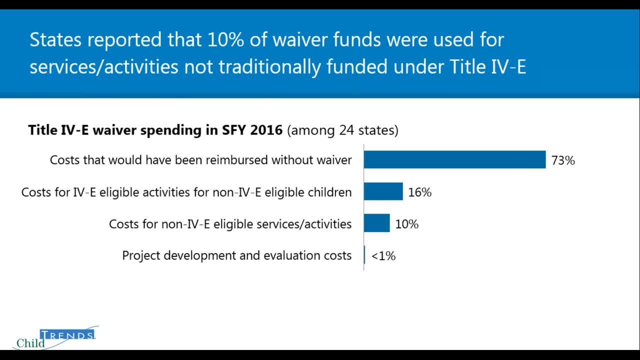 to help finance their waiver interventions. And also the federal IV-E waiver picture does not capture the possible benefits to the state of the welfare financing system overall. For example, even in states that are using a waiver to fund only IV-E eligible activities for non-IV-E eligible children. 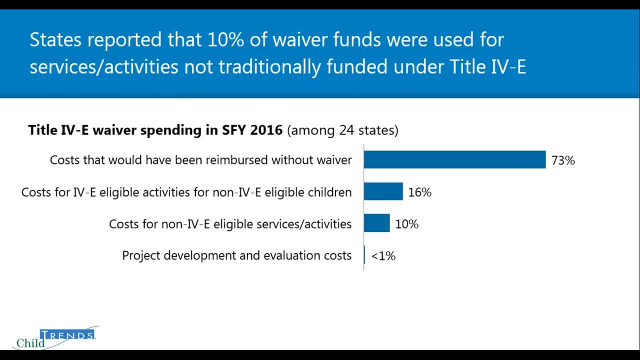 other dollars that would have gone to cover those costs are presumably freed up and might be used in other innovative ways. It's also important to note that, among the 27 states that reported waiver expenditures in 2016, California, Maine and Nebraska were not able to detail. 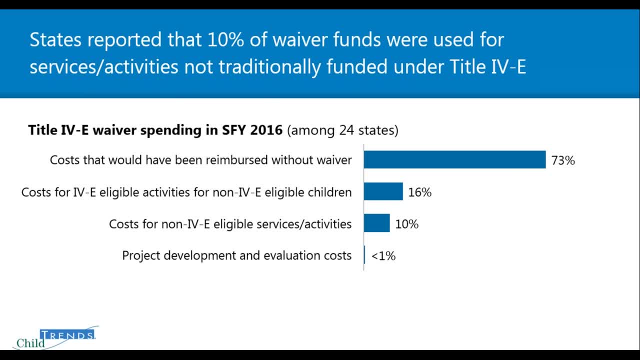 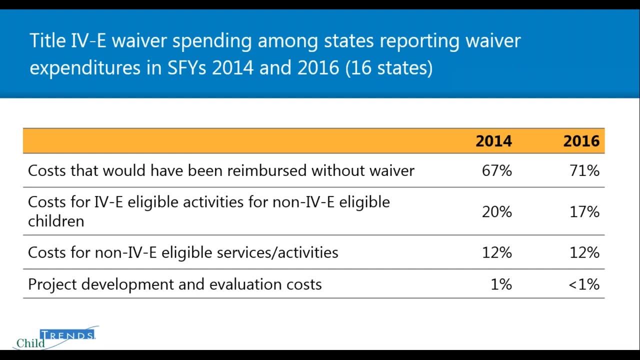 how they spent their waiver dollars, And since California is such a large state, the omission of its data may skew results, and so we recommend exercising caution when interpreting these results. We were also curious about whether how states spent their waiver dollars changed between 2014 and 2016.. 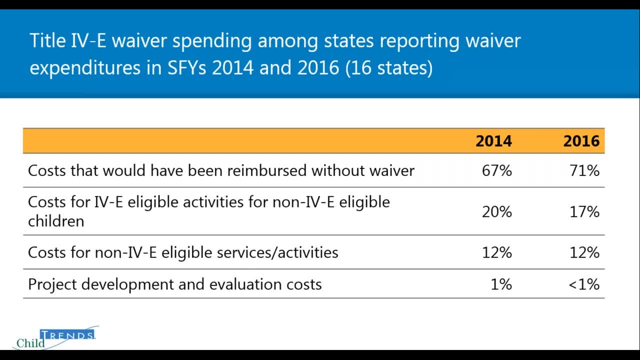 So among the states that reported waiver expenditures in those two years, the percentage of waiver expenditures that would have been reimbursed without the waiver increased a little bit and the percentage of waiver expenditures spent on costs for IV-E eligible activities for non-IV-E eligible children decreased slightly. 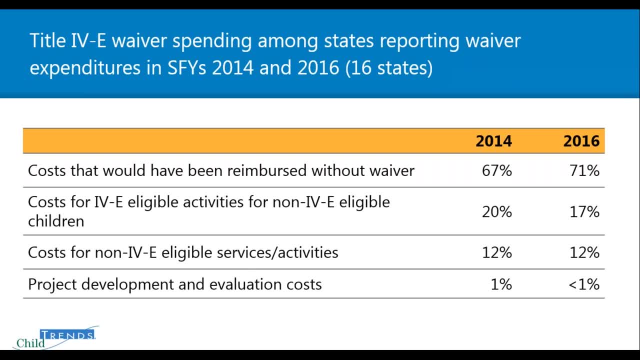 And this analysis that's shown on the slide here groups all waiver states together, but it's possible that the use of waiver dollars varies by when the state first started its waiver And, in fact, when we separated out the waiver states into three groups. 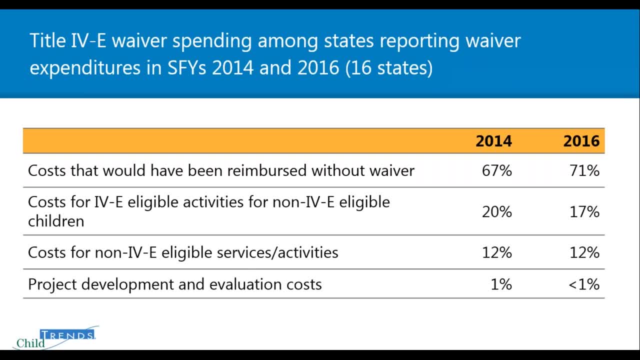 those that had a waiver the longest spent a smaller proportion of waiver expenditures on costs that would have been reimbursed without the waiver in that first category here. and the states that had a waiver the longest spent a greater proportion on costs for non-IV-E eligible services and activities. 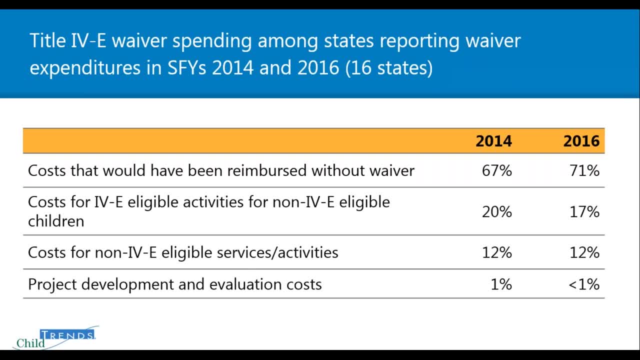 in the third category, And this difference may be a result of waiver states using their waiver interventions to reduce the number of children in care, which, over time, could reduce spending on traditionally eligible IV-E activities and increase spending on non-eligible activities. All right, 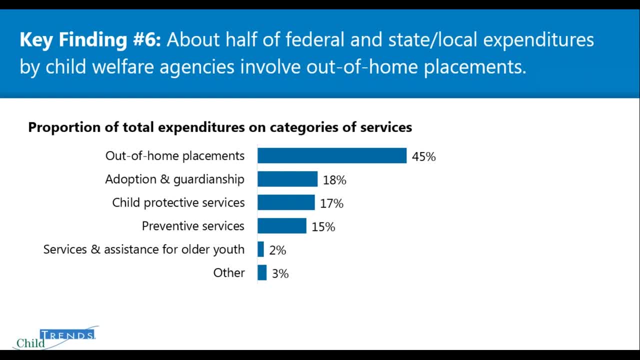 So key finding number six: About half of federal and state and local expenditures by child welfare agencies involve out-of-home placement, with smaller proportions spent on other services And, as you can see on this graph here, adoption and legal guardianship and home preventive services. 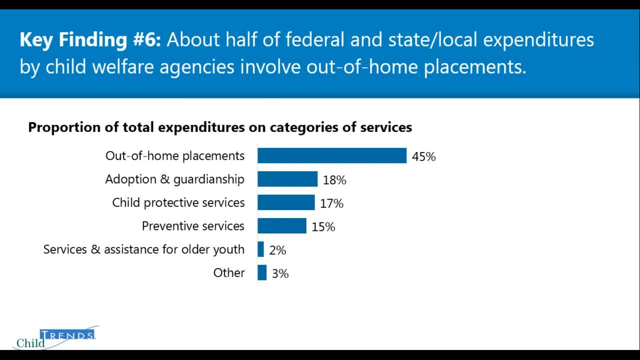 and child protective services each made up, about, you know, between 15% to 18% of total expenditures, And then a small percentage was used for services and assistance for older youth, And this slide shows the breakdown for federal and state and local funds combined. 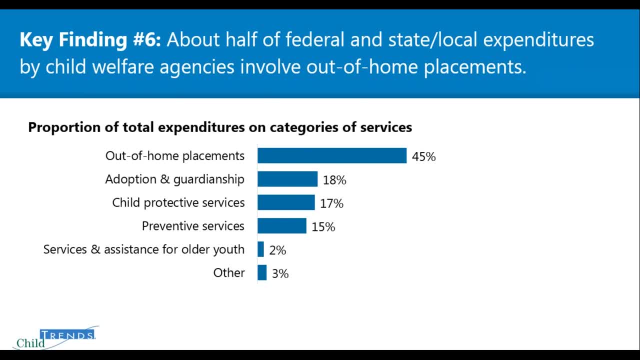 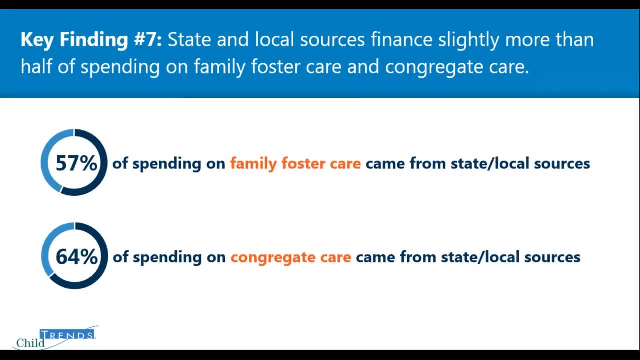 But if we were to break this out of, you know, federal funds versus the state and local funds, you'd see, you know you would see a similar picture, You'd see a similar pattern. So states also reported the amount of federal. and state and local funds that their child welfare agency expended on relative or non-relative family foster care and congregate care. So by family foster care we mean family-based placements like traditional or therapeutic foster family homes or relative foster care placements, for example. Then by congregate care settings we mean group homes, residential treatment centers, shelters, et cetera, And state and local sources financed slightly more than half of spending on both family foster care and congregate care. So as you can see here, 57% of spending on family foster care. 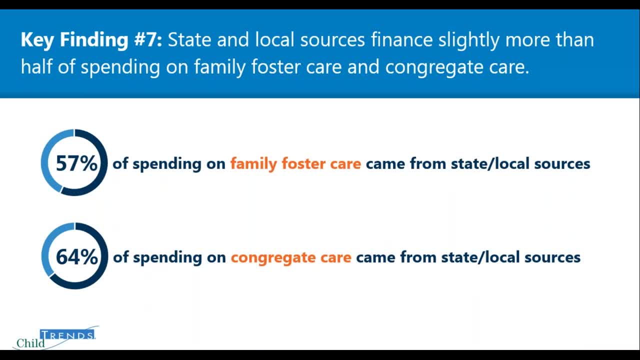 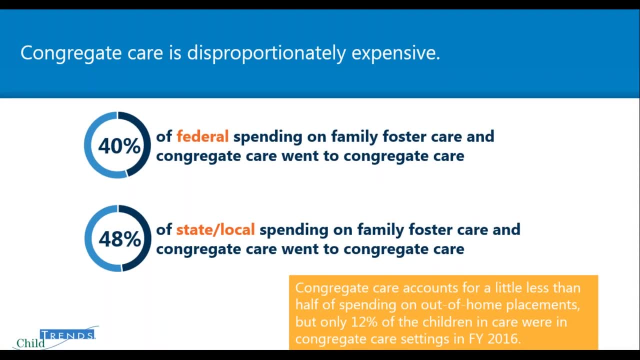 came from state and local sources, while 64% of spending on congregate care came from state and local sources. Then, when we're examining only federal spending on family, foster care and congregate care, we see that 40% of federal spending on these placement settings was spent on congregate care. 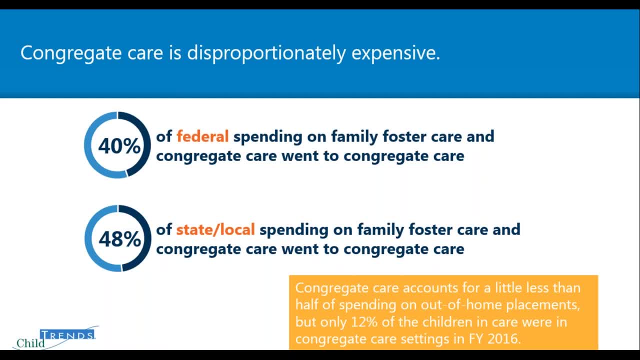 And then, when examining only state and local spending on these placement settings, 48% of state and local spending on these placement settings is spent on congregate care. So this information about spending on out-of-home placement settings shows us that congregate care is disproportionately expensive. 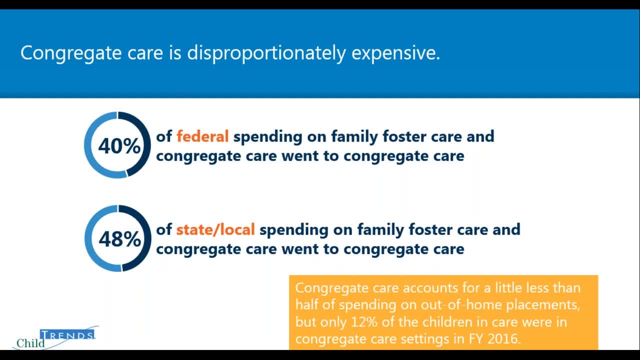 And that's not shocking to anyone. I think that's well documented. but this helps put some numbers to that understanding. As you can see here in this orange box here, congregate care accounts for a little less than half of spending on out-of-home placements. 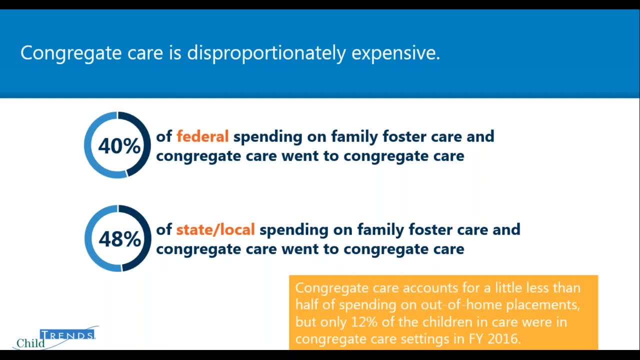 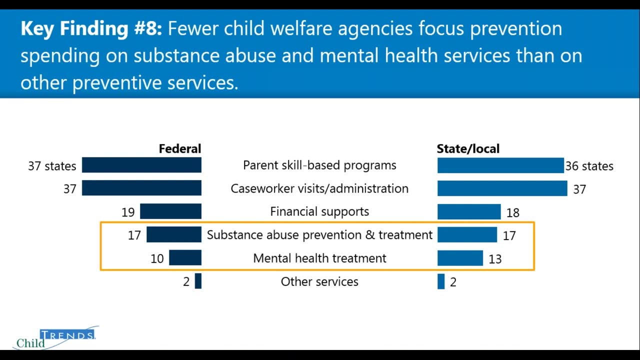 but only 12% of the children in care were in congregate care settings in fiscal year 2016,, which helps us understand just how disproportionate the cost is. All right, so key finding number eight is that fewer child welfare agencies focus prevention spending. 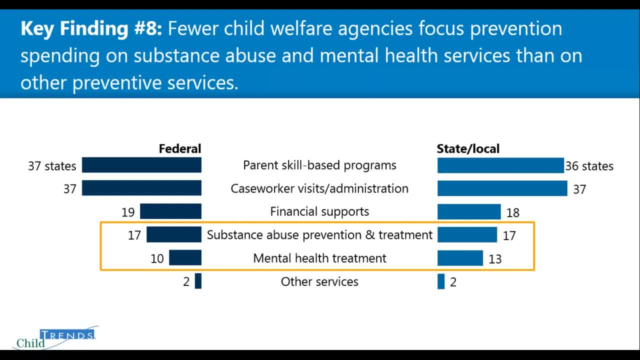 on substance use and mental health services than other preventive services. This year, we began asking states about their spending on different categories of prevention services, So this is one of the new questions that Christina mentioned. at the beginning, States ranked the top three categories of preventive services. 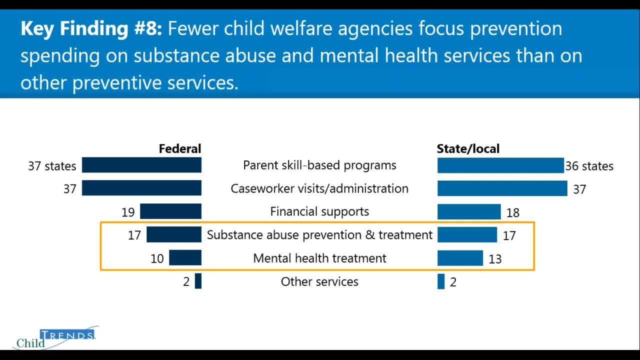 for which their child welfare agencies spent federal and state and local funds, And the figure here shows the number of states that ranked each preventive service in their top three. So the top services in 2016 were parent skill-based programs, caseworker visits and administration. 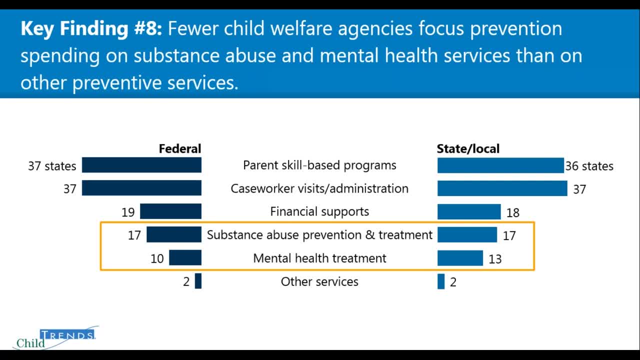 which included information and referral services and financial support such as assistance with transportation, housing, childcare and more. And there are a relatively small number of states in which the child welfare agency focuses its prevention spending on substance abuse and mental health services. 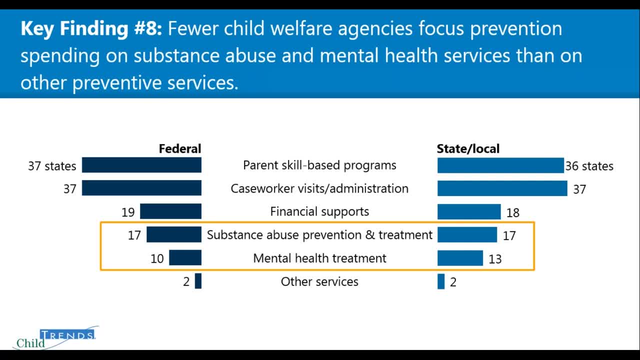 And this finding is important given the need for these services among families involved in the child welfare system, as well as the ongoing opioid crisis that's straining many child welfare systems across the country. It's also important to note that, while child welfare agencies may not be focusing their prevention spending, 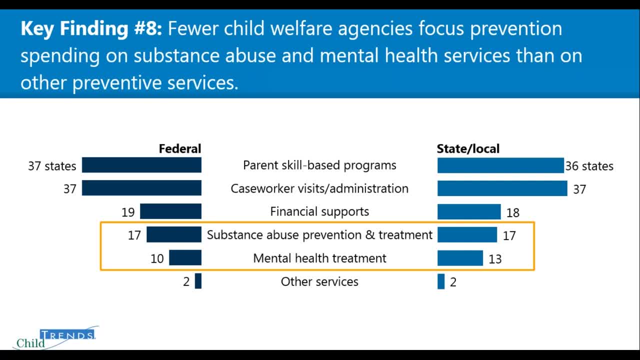 on these programs. it's possible that the child welfare agencies in those states partner with other agencies, such as health departments, to fund such services. So this is not meant to mean that those services are not being provided. They are just not being funded by child welfare agencies. 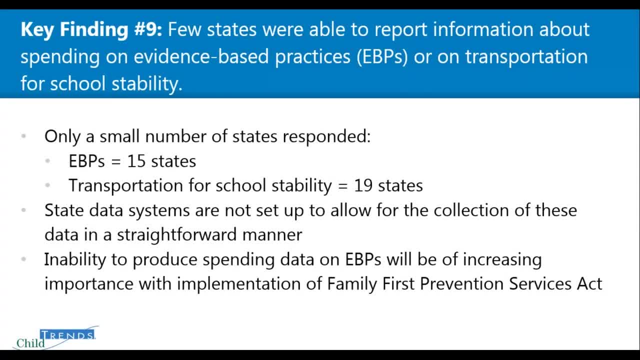 All right, and our last key finding is related to spending on evidence-based practices and transportation for school stability. On this year's survey, we asked questions about these topics and they were new questions this year, But only a small number of states responded to these questions. 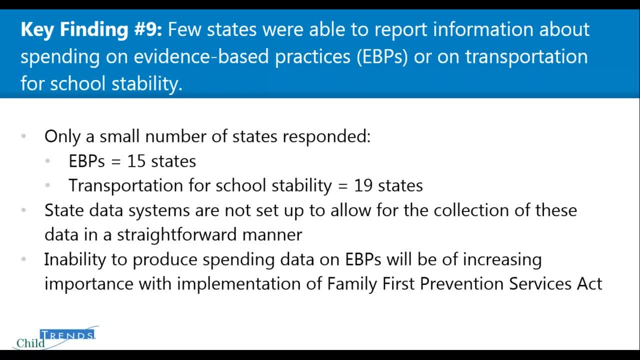 so we're unable to report national results. Our assessment is that state data systems are simply not set up in a way that allow for the collection of these data in a straightforward manner. So, for instance, costs for transportation to maintain school stability may be bundled with other costs. 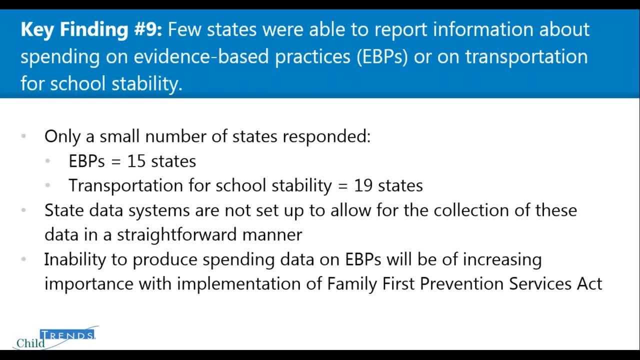 like a foster care maintenance payment if foster parents are the ones providing the transportation, And that makes isolating transportation costs difficult. So while we can't produce national findings related to spending on EBPs and transportation for school stability, the fact that so many states 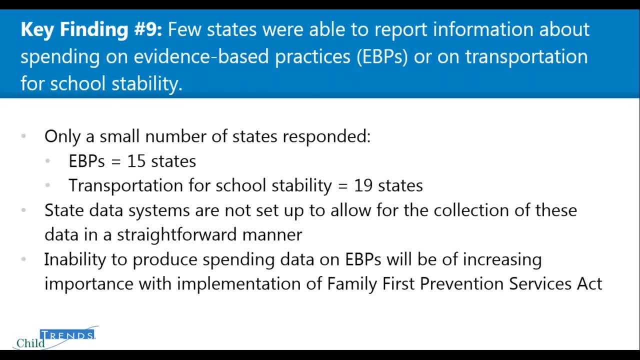 struggle to report this information is significant in itself. In particular, states' inability to produce data on spending on evidence-based practices will be of increasing importance as states begin implementing the Family First Prevention Services Act, since that law requires states to track spending on EBPs. 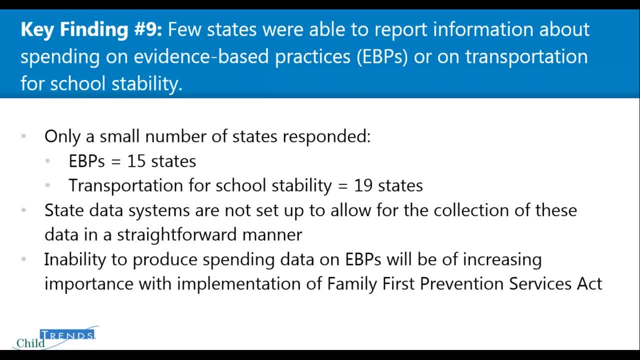 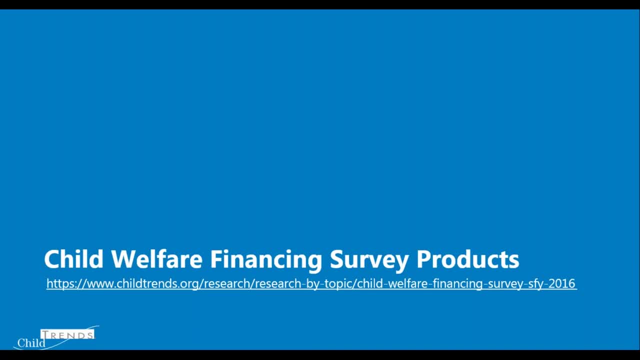 and promising practices in certain circumstances. All right, so that's our discussion of the key findings, And before we go on to answering questions, I'm just going to give you a preview of the additional products that we have on our website. So while I'm doing that, 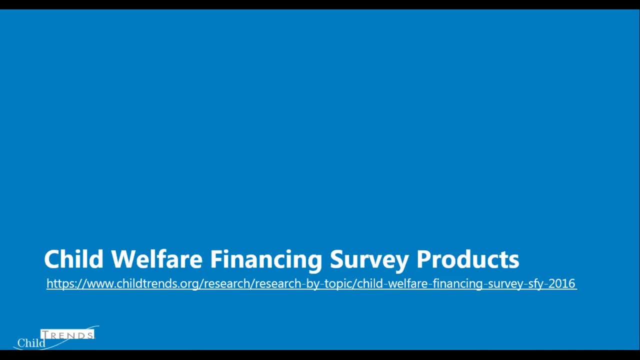 if you have questions, please enter them into the chat box or the questions box and we'll answer those momentarily. So all of these products that I'm going to give you a preview of are available on the Child Trends website. I have the link here. 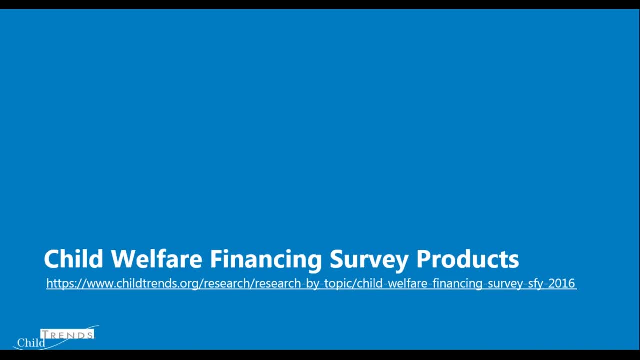 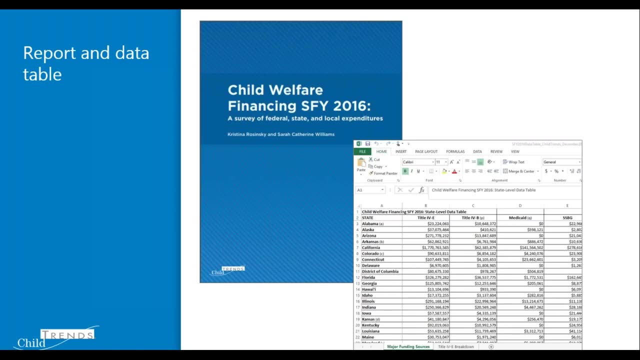 but if you Google Child Trends, Child Welfare Financing, the report will come up. So first off is the full report, which includes an executive summary, a detailed presentation of the findings, a discussion and appendices with state-level data. So when someone had asked the question, 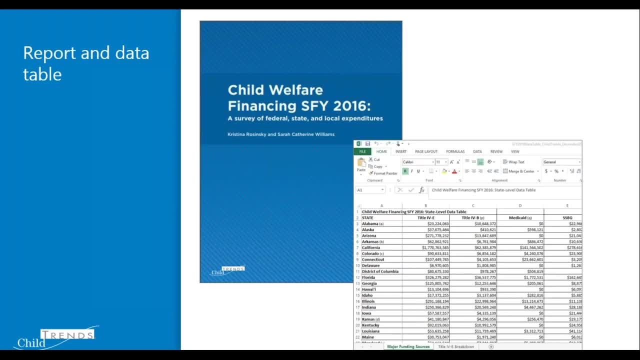 of whether or not we have state-level expenditures available- and we do. they're available both in the report and in another resource that I'm going to highlight in a moment. For those of you who are data nerds like me, we also have an easy-to-use. 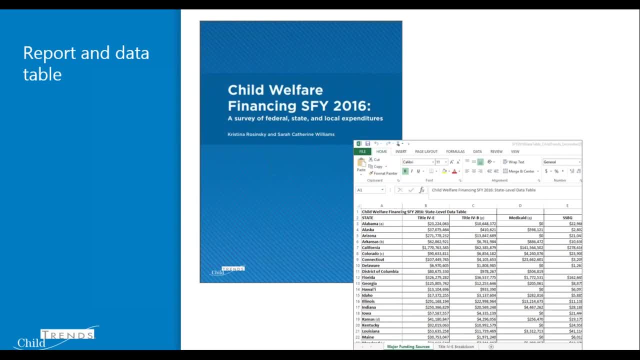 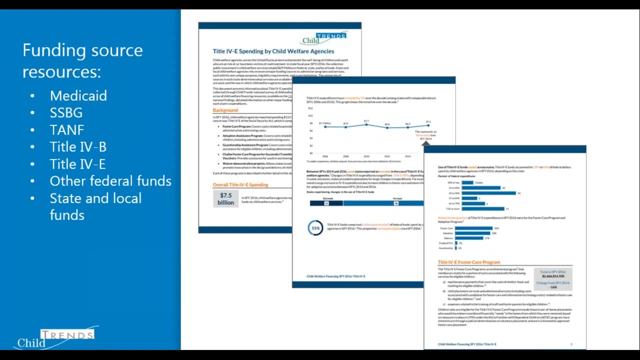 state-level data table in Excel that you can download and play around with. So both of those are available on our website. And then, if you're interested in learning more about a specific funding source, you can take a look at our funding source fact sheets or resources. 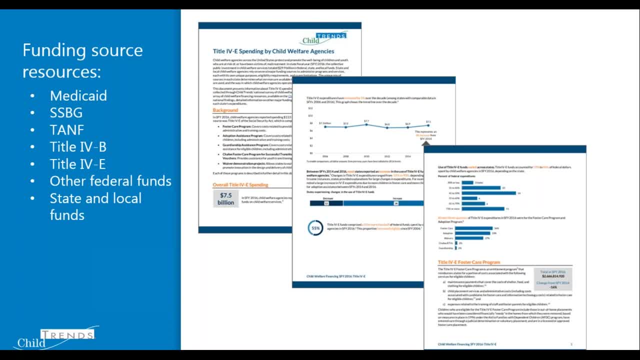 Each one breaks down one of the major funding sources down a little further than in the main report And they're great for those of you who are new to child welfare financing to get a better understanding of each of the major funding sources. But these resources have more graphics. 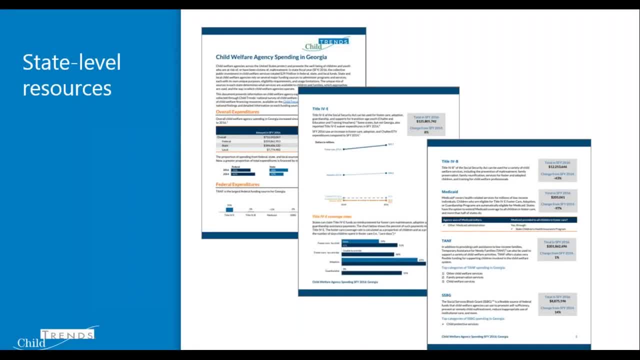 and that kind of thing. And then, finally, if you want to know more about funding in a particular state, in addition to the information and the appendices, we have some state-level resources as well, And these resources provide all of the available information. 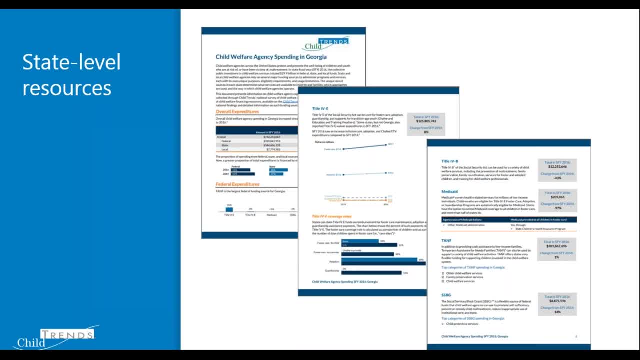 for each state in one place, whereas the appendices and the data table. those are good for making comparisons amongst different states. But if you're really wanting to focus in on one state, these are great, because it has all of the information about that state in one place. 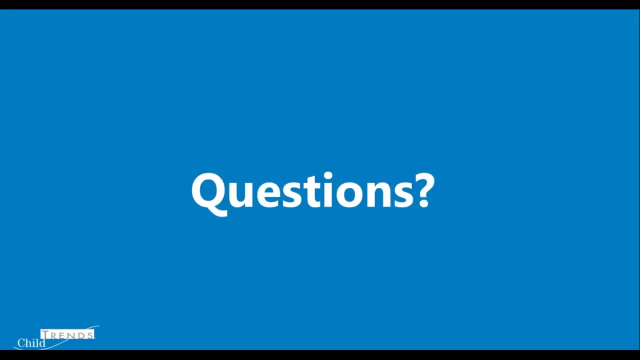 So now we are going to stop for questions And I'll just say we may not be able to answer all of your questions, but we'll try and follow up with you if we don't get to your questions And since there are so many of you on the webinar, 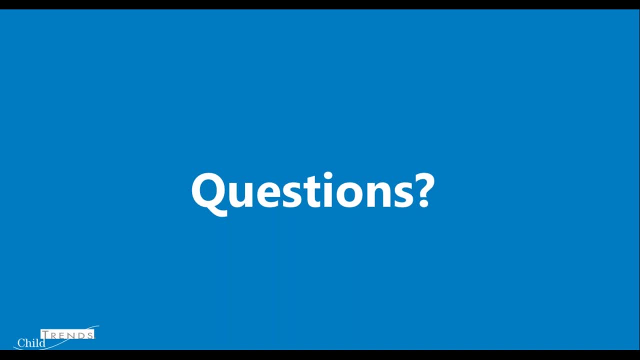 instead of unmuting folks, we're going to read questions from the question box and then answer them, So we've had a couple come in so far and feel free to type in your questions in the question box. Our first question comment is from Carolee Morano. 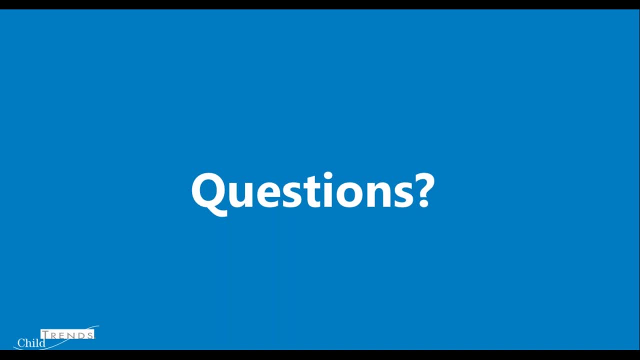 Carolee made a comment around how there has been a shift. She's seen a shift in her organization where there's been fewer referrals to congregate care replacements and with a priority being more focused on family-based settings and family preservation, prevention services, that sort of thing. 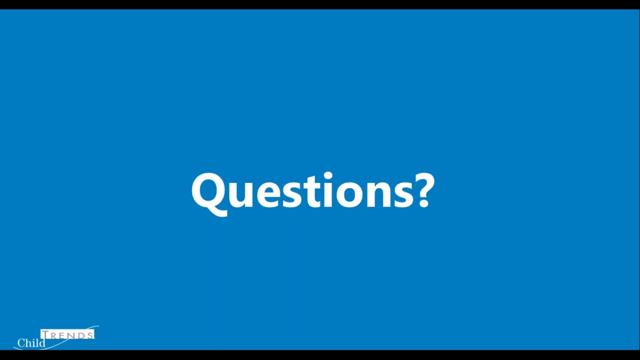 And she asked if the 5% increase in child welfare expenditures is related to that shift in priorities. That's a good question And, of course, like we shared earlier that the reasons behind these trends are complex And a piece of it could be the shifting priority. 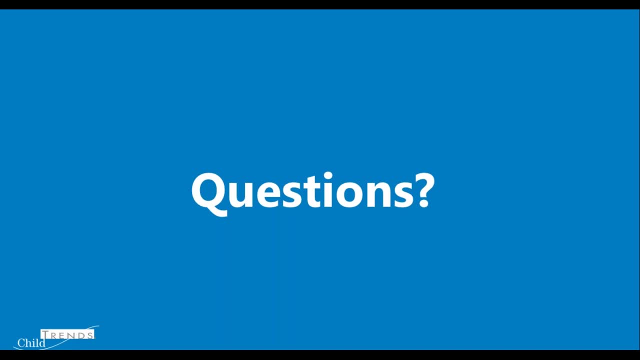 more towards family-based settings, more to upstream services, That would, in my mind, drive expenditures down. It wouldn't drive expenditures up per se, But again, the story is complex And if more families are being served, even though fewer children are going, 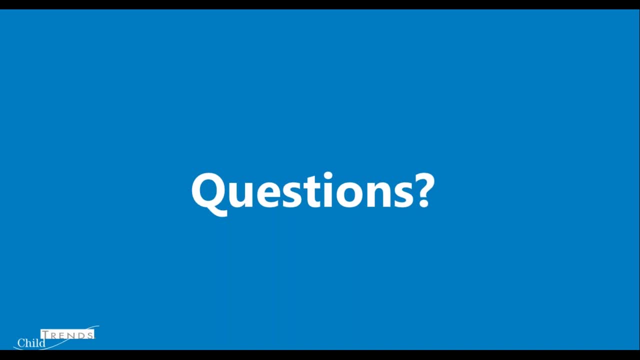 to congregate care replacements that could contribute to increases in expenditures. And Carolee also had later in her comment a note around how the slide around showing congregate care and how it's disproportionately expensive. she noted that it's one thing to say. 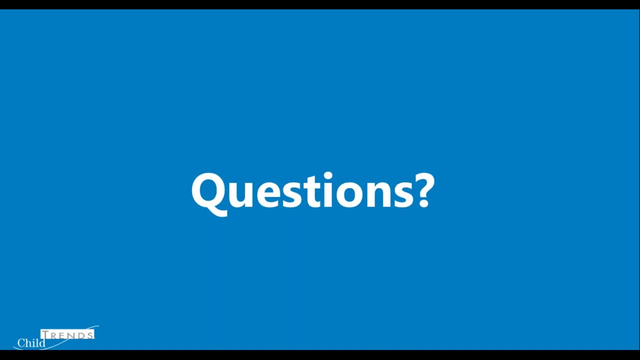 that it's costly, but do we know if there's a benefit in terms of the outcomes that justifies the cost, And are those sorts of things being looked at? I think that's a really good point. That's not something that our survey looks at. 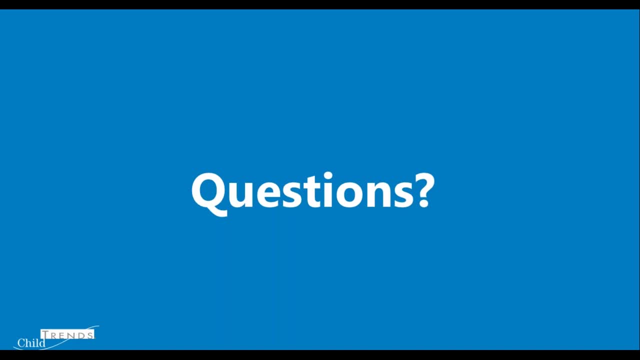 We're just focused on the expenditures and what the money is being spent on, But that's an important consideration to keep in mind. It's not all about doing things more cheaply. We have to keep in mind what's best for that child and family too. 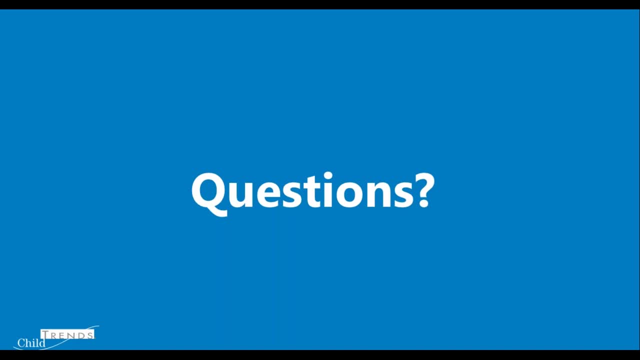 So that was Carolee's comment. I'm going to pass this one to Sarah Kass and I'll ask this question of you from William Thorn: Do you have resources or information on tribes? We do not have information or resources on tribes. 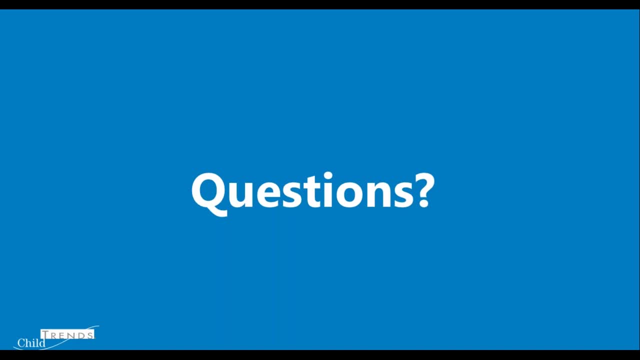 The survey is sent to state child welfare agencies. It's outside of our current survey so we don't have that information, But we do have resources on the state side of our current scope to look at tribes and their specific expenditures, But that's something that we always have. 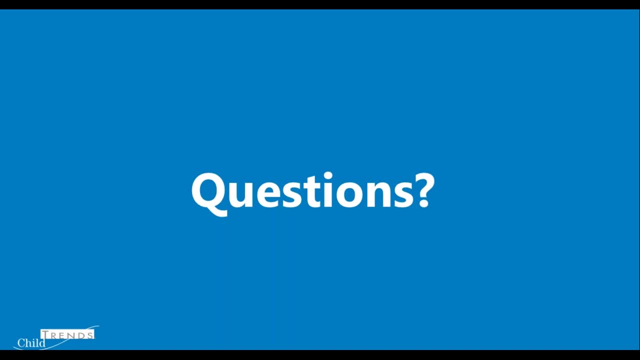 in the back of our minds were additional resources to look how it's available. Great. So I just want to put out the call again for folks to add their questions to the question box. We got a comment from someone else mentioning that it's designed to be cost neutral. 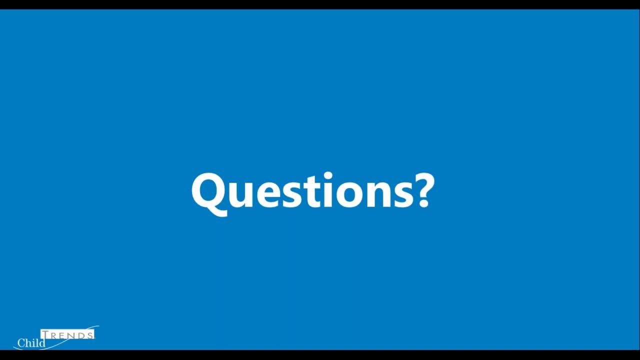 over the term of the waiver. Thank you, Charlie Ferguson, for noting that, But do any other folks have questions or comments that they would like to make, And, if so, you can use this time to enter the question into the question box. 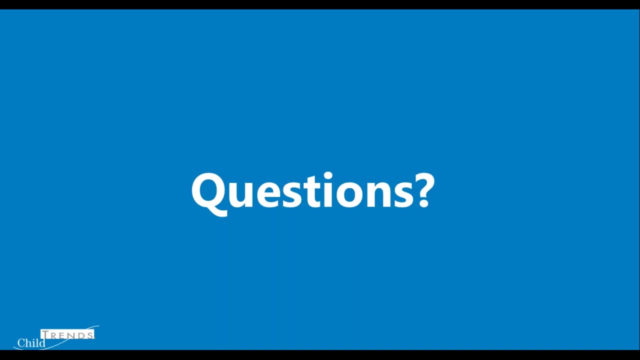 We'll give folks a minute or so to kind of think up of their question and type it in. Looks like Carol Lee may be in the process of submitting a follow-up question, so we'll give her a moment. So Carol Lee's follow-up question. 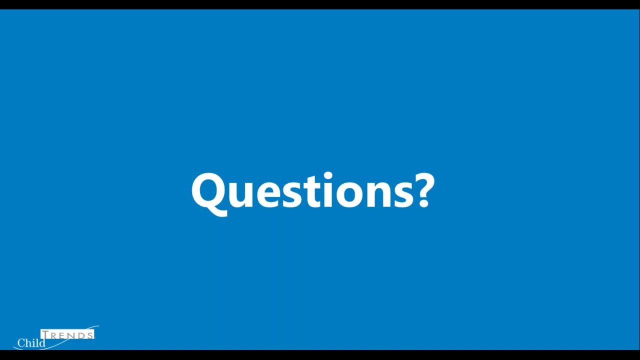 around the shift away from congregate care and prioritizing more family-based settings. she indicated that there is concern that that shift may have an unintended consequence of shifting the burden of services and costs from the child welfare system to the runaway and homeless youth system of care. 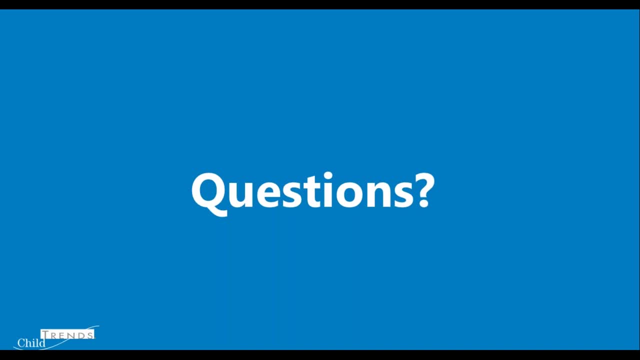 And there's also a concern that there may be an unintended consequence of shifting the burden of services and costs to that system of care And she asked if that's being looked at. And so again, another great point around, kind of the kind of the big picture. 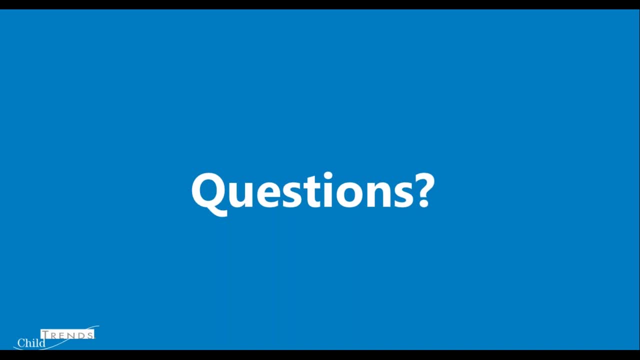 of you know how this population is being served. Our survey is just focused on child welfare agency expenditures. We don't look at, say you know, for example, there's a lot of interest in the education system and health system and their spending on this population. 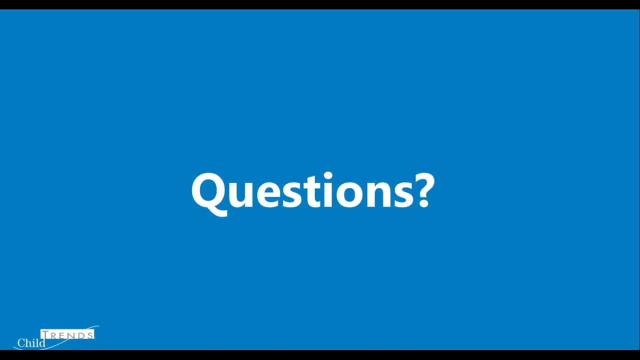 Likewise, you know runaway and homeless youth system of care as well. You know there are lots of agencies and entities that provide services to this population, You know, while they're in foster care and then later in life as well. But our survey is just focused. 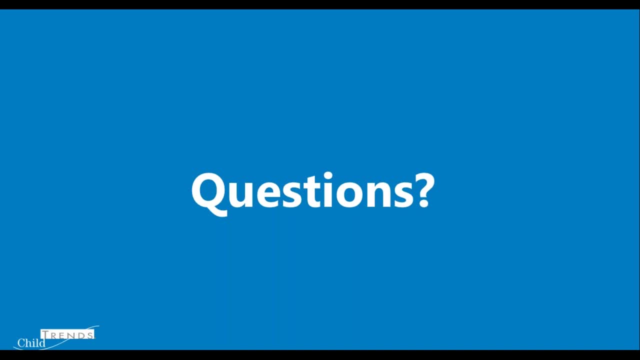 on child welfare agency spending. So unfortunately, no, we don't. We don't have a sense of any kind of shifting costs that may be going on. Yeah, And so Aubrey Edwards asked if this level of analysis is available by state on the website. 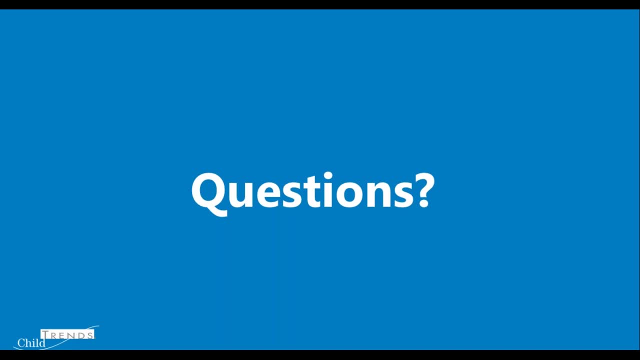 And it is, And the The appendices of the main report has. you know pretty much, for I believe it's for every, Well, almost every question asked. we, you know, give each state's response in the appendices, including you know. 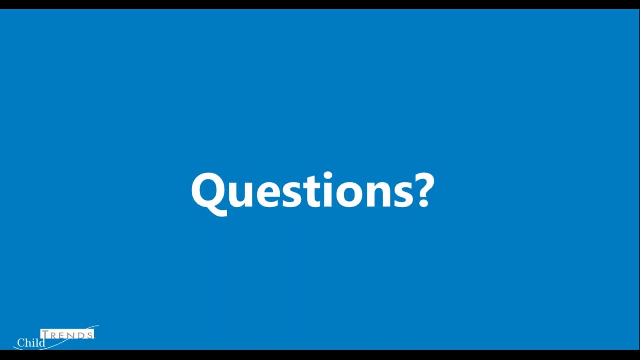 percent change from one year to the next. So if you're interested in the state-level data, you can take a look at the appendices in the final report as well as the state-level data. There's a lot of resources. There's one for every state. 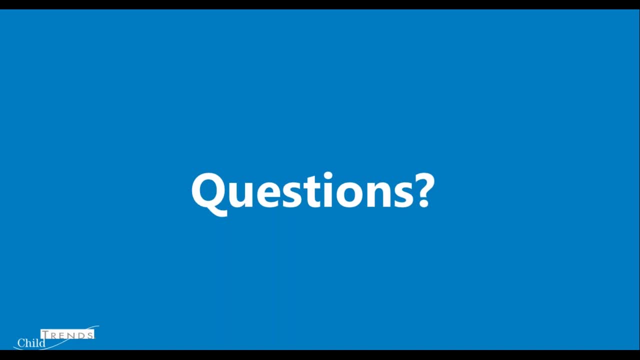 Mm-hmm, And if there's anything that you can't find that you really are interested in, justyou can e-mail us and we'd be more than happy to provide you what we may have. There is a lot in the appendices. 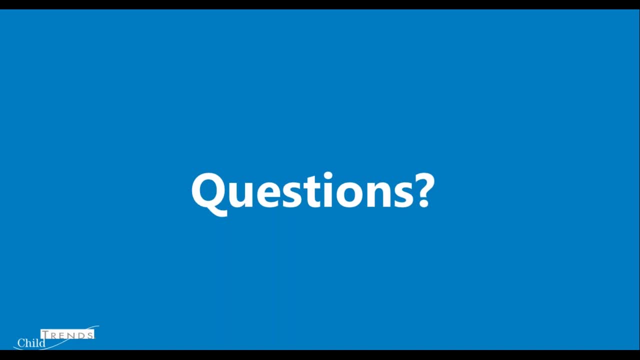 So if you're having a hard time finding it, you can always shoot us an e-mail. So Jennifer has a question about whether we have any thoughts on the funding impacts of the Family First Prevention Services Act for waiver states. That's a very timely question. 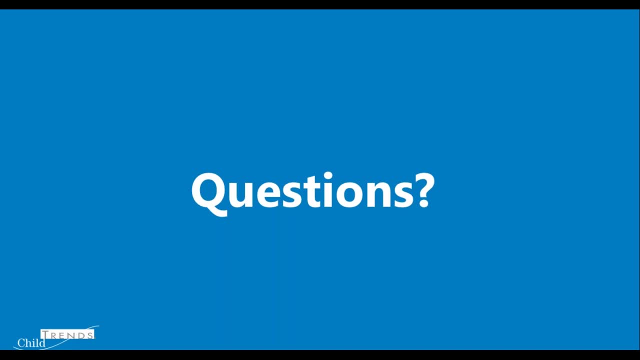 And so you know, as I mentioned in the waiver part of the conversation, that with the end of the waivers it's expected that the waiver states may lose more than $300 million in federal IV-E funds, But of course, if the states implement. 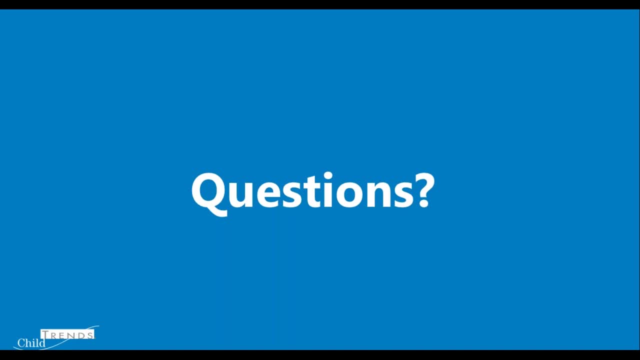 the Family First Prevention Services Act in its entirety, that could help you know, mitigate and help with that transition a bit, because a lot of the waiver interventions that states are implementing are prevention services that could be eligible under the Family First Act And so that transition to Family First. 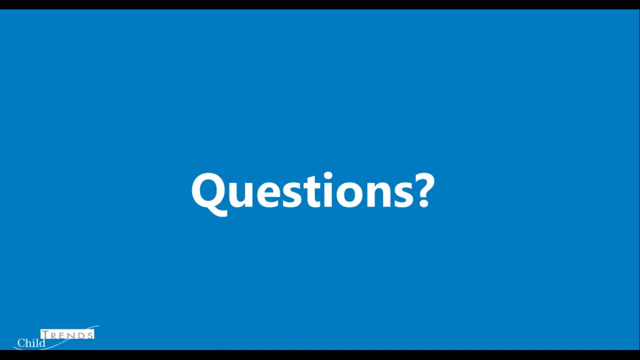 kind of may make up for kind of some or all of what the states may lose under the waiver. So we've answered all questions submitted so far. If you have any other questions, feel free to submit them now. We'll pause for a moment. 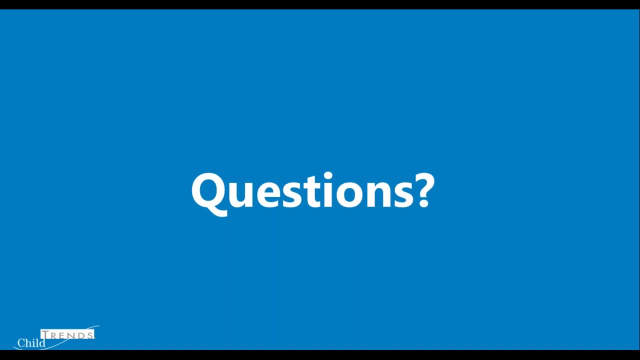 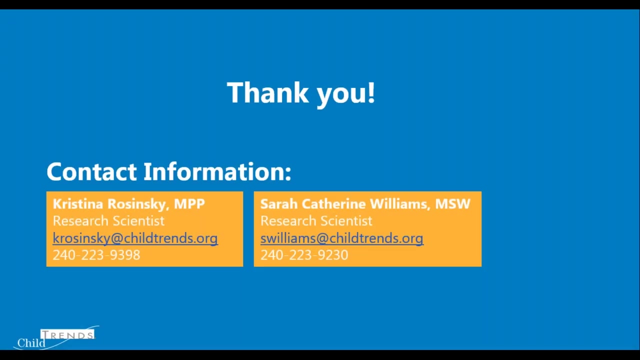 to give you a chance to type them in. All right, so we're not seeing any other questions. Oh wait, I spoke one millisecond too soon. So, Andrew Kim, he submitted a question saying I'm sorry I missed the part about the substantial decrease. 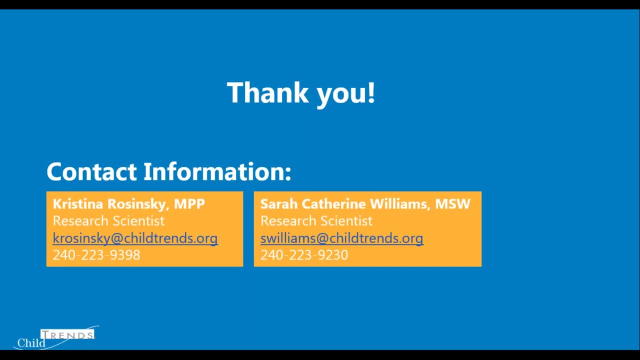 to Title IV-B in Medicaid. Could you briefly explain why? Yes, I'll try to briefly explain why. That's the challenging part because it is quite complex, But in kind of a broad brush, kind of nutshell, the trend in IV-B has gone down. 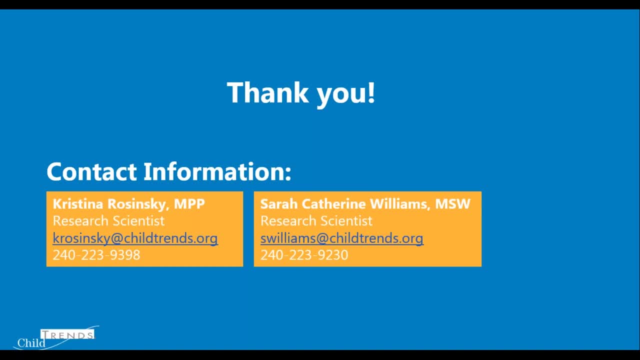 because of one sequestration. Sequestration affected IV-B- Part II- a bit. It wouldn't account for the full 29% decrease in IV-B, But the larger piece of the story around IV-B is kind of how it's set up. 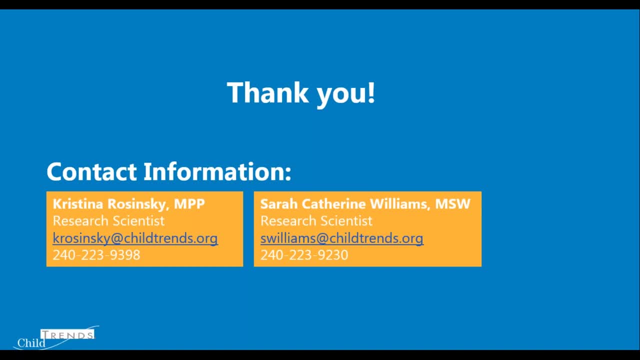 Title IV-B, Subpart II, is set up in a way where there's a set amount of funds And before funds are made available to child welfare agencies for services, there are particular programs that are funded through set-asides. So of the total amount there's some funds. 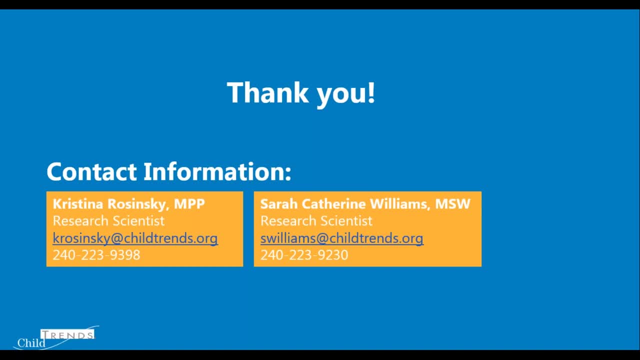 that are set aside for the court improvement program, for regional partnership grants and some other things as well, And after those set-asides are taken into account, then what's left over is available to child welfare agencies for services, And what we've seen is that over the past decade, 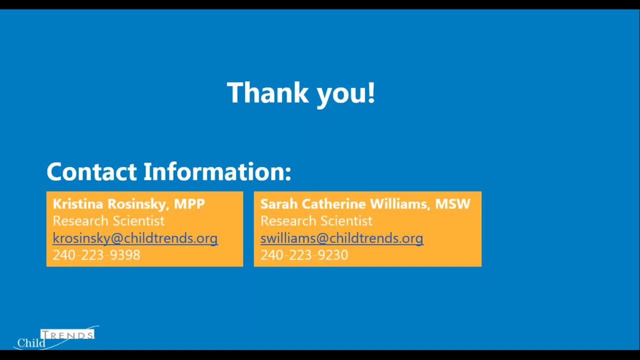 some of those funds, some of those set-asides. the amount of those set-asides has increased And so as those set-asides increase, the amount left over for child welfare agencies goes down. So that's the kind of big-picture story around IV-B. 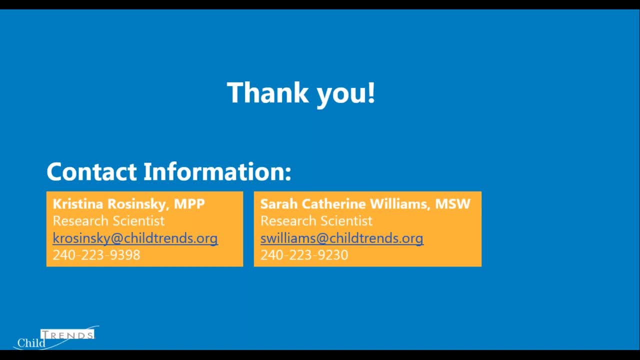 As for Medicaid, we saw a 46% decrease over the past decade. And again, specifically, you know child welfare agency spending of Medicaid. The story there is around, you know, shifts in how child welfare agencies use Medicaid. So, for example, we've seen that over the decades. 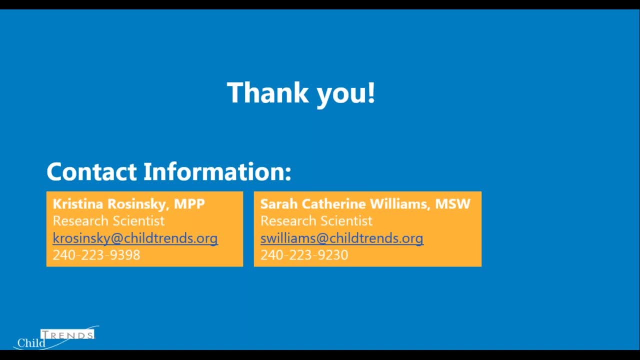 fewer child welfare agencies reported that they use any Medicaid dollars at all And there's also been shifts in like sort of administrative, of administrative nature with Medicaid, where child welfare agencies are shifting Medicaid-funded services to another agency or transitioning from fee-for-service. 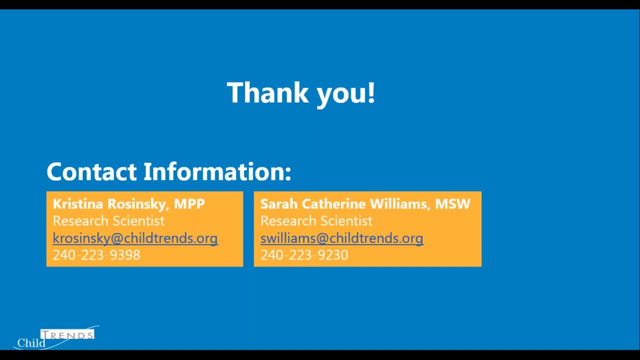 to managed care systems or bundling or unbundling Medicaid services And those sorts of things can impact how you know Medicaid is accessed and which agency is responsible for paying for Medicaid costs. So that's sort of the summary of IV-B and Medicaid. 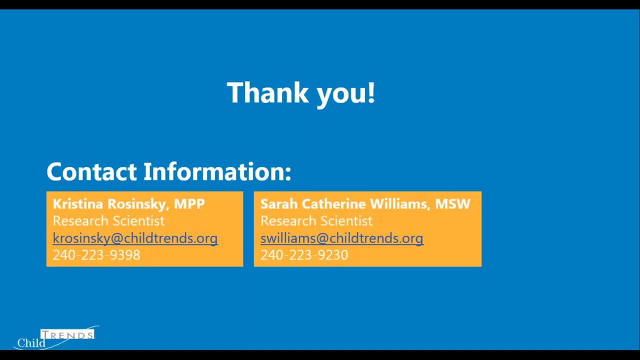 and why those have decreased. Charlie Ferguson has asked a question around. can you clarify your statement about waiver jurisdictions losing funds in the source of the dollar amount you provided? I would be happy to Charlie, So I'm going to actually go back in the slides. 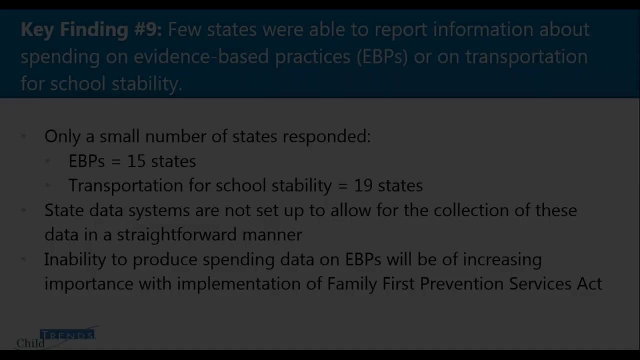 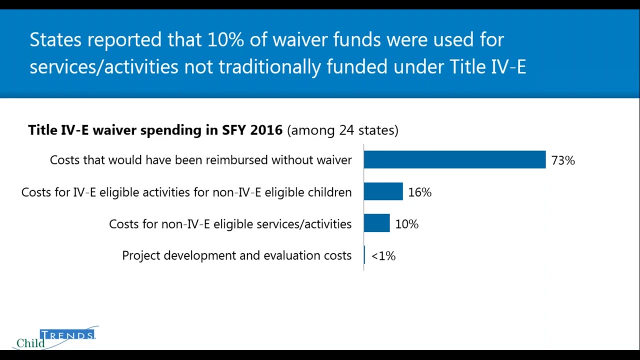 Sorry for the whirlwind. This will be a good refresher in case anyone has any questions, because the slide is helpful in illustrating this. So the way we came up with that $300 million estimate is that we asked states. you know how they have waivers. 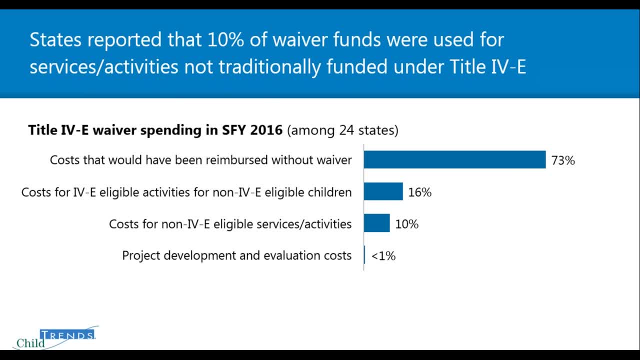 How do they use their waivers? And the first category here: costs that would have been reimbursed without the waiver. you know 73%, you know even after the waiver they would still get IV-E for that. It's those other categories, the costs for IV-E eligible. 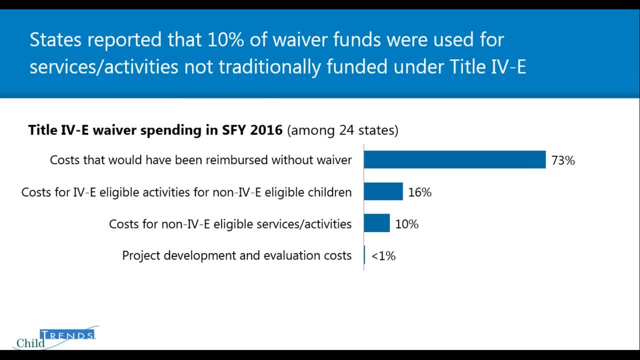 activities for non-eligible children and costs for non-IV-E eligible services and activities, That 26% those two categories combined. we take that 26% of the total waiver expenditures reported to us by the 24 states that were able to report this breakout. 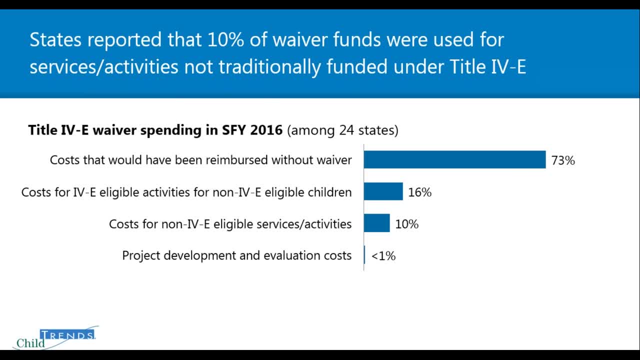 And so that 26% of the total of these 24 states is that $300 million. One caveat that I mentioned before, but it's worth reiterating here, is that California is not included here also Maine and Nebraska, but California is a very large state. 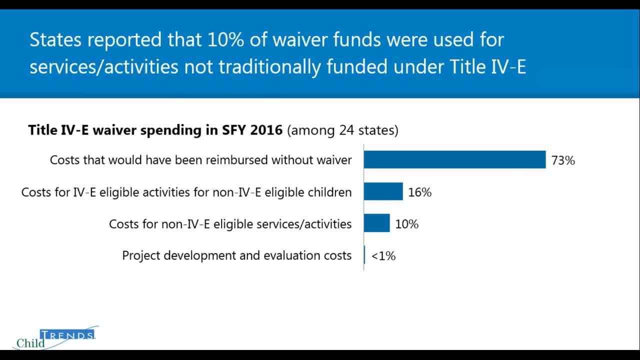 And so when we cite that $300 million estimate, that's a sort of lowball estimate, because if California were included that would increase quite a bit. So we basically just use that as a way of illustrating how the end of the waiver may impact states. 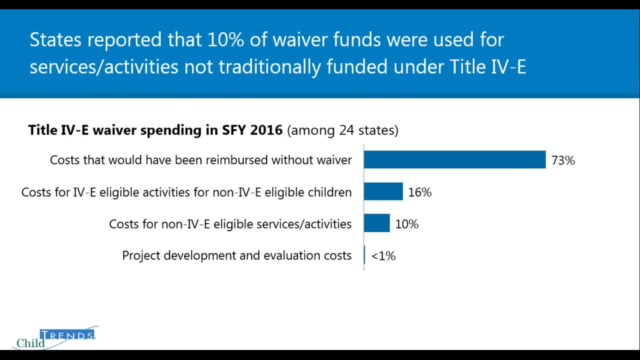 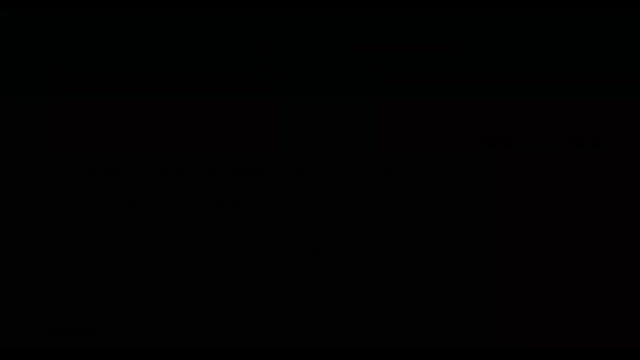 And our calculation here is that the end of the waiver would result in a loss of more than $300 million in IV-E funds. But, like I was mentioning earlier, the implementation of Family First will help mitigate some or all of that. So I'll go back to the final slide. 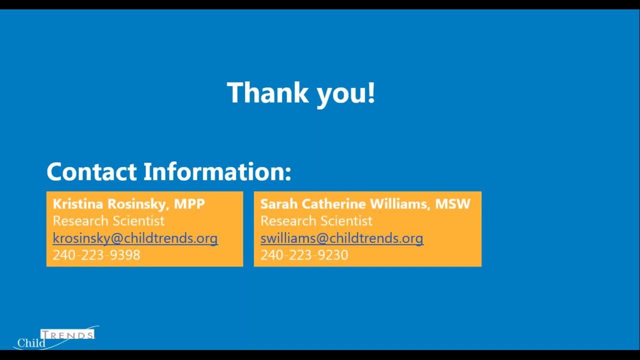 Any other final questions? All right, I'm not seeing any others come in, So if you have any questions that come up after we conclude, our email addresses and phone numbers are up on the screen here. We will be posting these slides on our website. 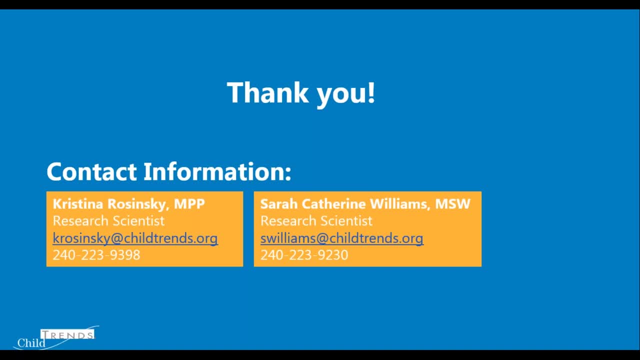 after today's webinar And, like I mentioned at the beginning, we tried to record. We hope it recorded. We did have some technical difficulties, so we apologize if the recording doesn't go through, But if it was successful that will be posted on our website. 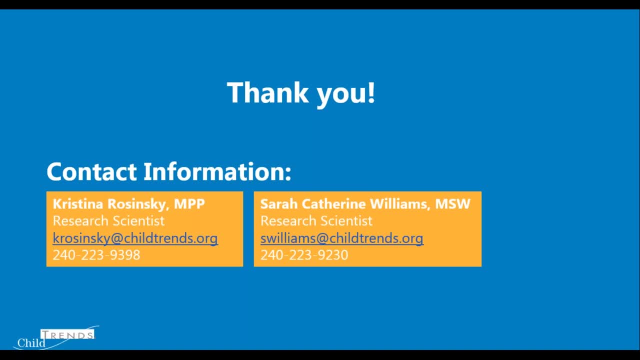 alongside these slides as well. So thank you everyone for joining. I hope this was useful and informative And again, feel free to reach out to us with any follow-up questions or comments that you may have. Have a great afternoon, everyone.